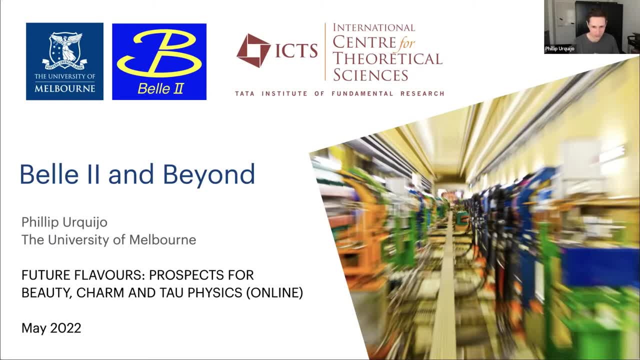 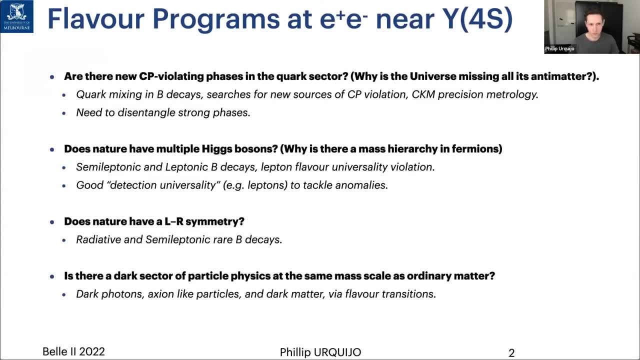 in the near future with the super-KB collisions as pictured. Typically, when it comes to a long-term flavour program, you need a long-term vision, and we usually drive that with open questions, and you might be able to apply some of these to other experiments, for sure. 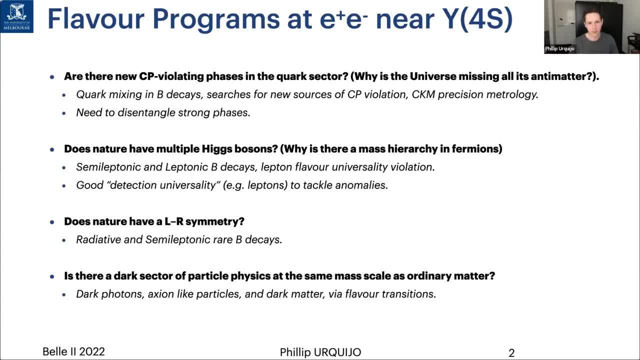 but I think these ones are all really quite applicable to you know a lot of the things that we're looking at. So we're looking at, for example, E plus, E minus near epsilon 4s. So, firstly, are there new Cp-violating phases in the quark sector? 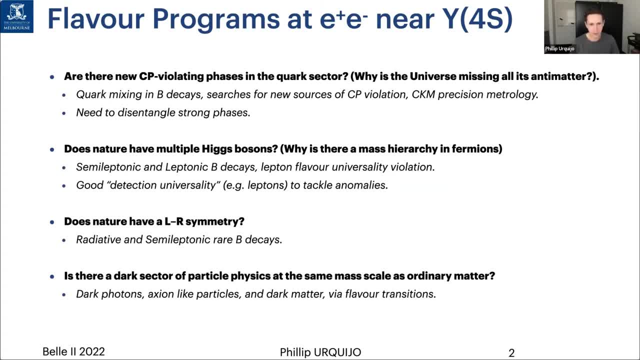 We know the universe is missing all its antimatter, but we don't know why. We're looking at quark mixing in beta-Ks- new sources of Cp-violation. We're using CKM- precision metrology- and, from a phenomenology perspective, we also need to. 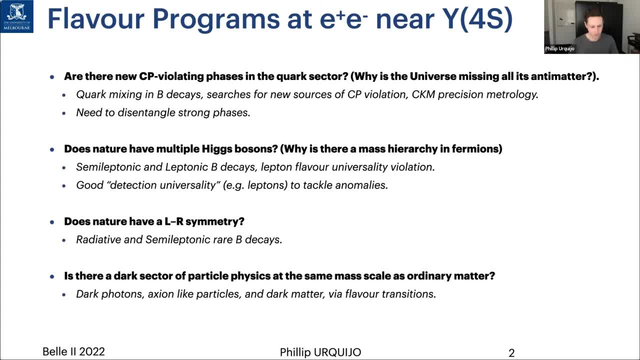 disentangle strong phases. So we need to know what we're doing. We can't just make a direct measurement, We need to really understand the mechanisms that can give rise to Cp-violation. Secondly, we want to know why the universe has three families of fermions, these three copies of things with different masses. 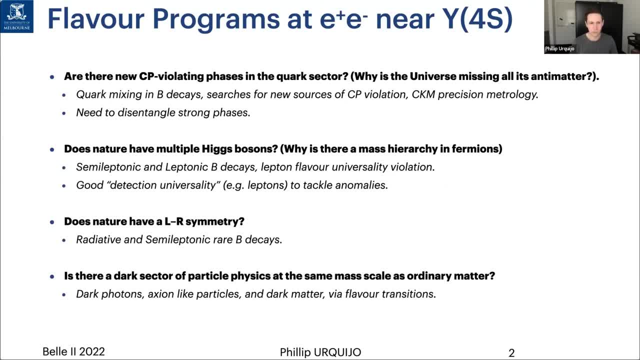 but are essentially the same. Maybe it's got something to do with having more Higgs bosons. A type of measurement that you can do to look for this is: you look for a lepton flavour universality violation and this is shown up as a fairly significant. 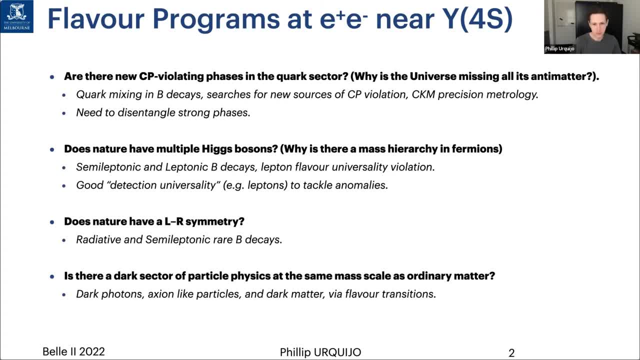 hint or anomaly years of new physics in more recent years. I'll go through some that are being worked on with Bell2.. The third one is the, the W. It's left-handed. For some reason we have this chiral structure in the standard model in nature, from what we can see. We can't easily explain why. 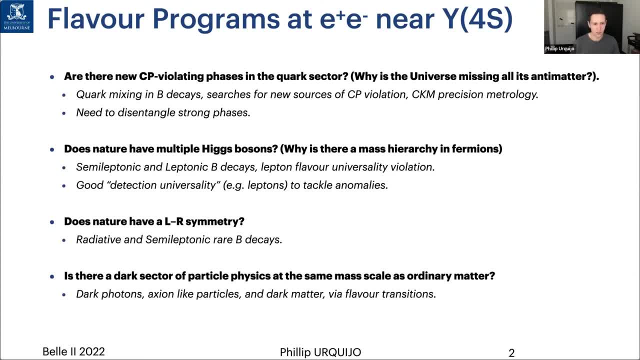 Perhaps there is a right-handed counterpart that is much heavier, and there are really good ways to do this through studies of weak decays of bees. And another thing that's become really popular in more recent years is the prevalence of searches for dark sectors and the concept that dark matter could be rather complex and involve interactions. 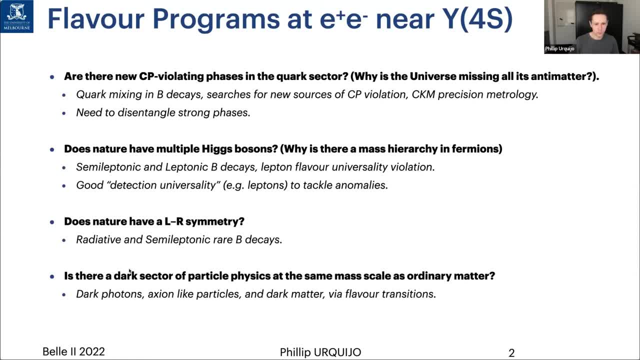 with ordinary matter in a very feeble way. So we're looking for feeble type of interactions: dark photons, axion-like particles and dark matter via flavor transitions. This is a picture that's been shown in the last couple of years. This is a picture that's been shown in the last couple of years. 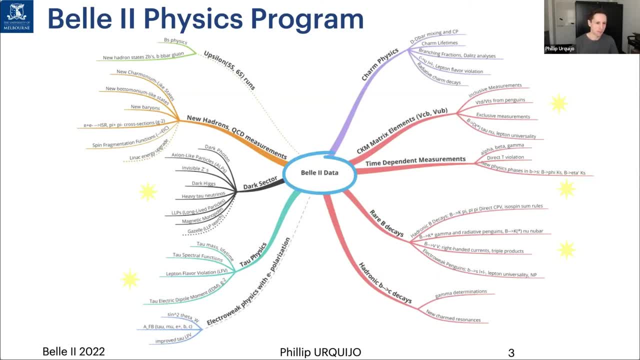 taken from the Bell2 SNOMAS program associated to upgrades and the physics program in general. You can see there are many, many arms from many arms corresponding to areas of physics analysis. I'm going to cover a few, but you can continue on and do study. 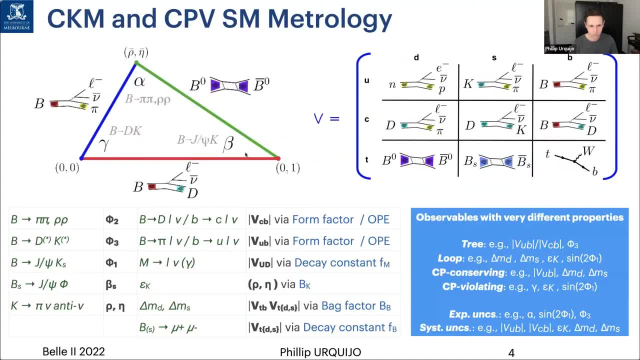 many more areas of physics if you're interested. So, coming back to CKM metrology, This is kind of the bread and butter physics of a bee factory. The principle is that we're measuring the CKM matrix elements and we're measuring the amount of CP violation in 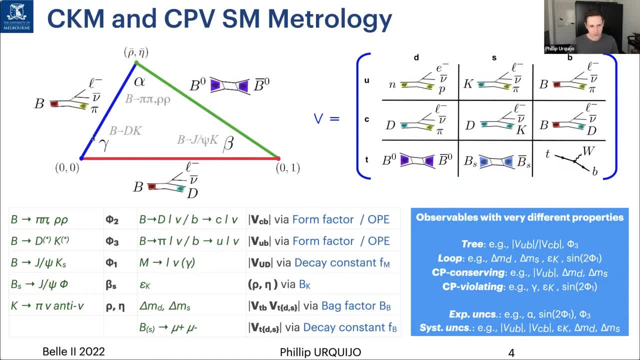 the standard model, We can measure the amount of CP violation by performing direct. by performing measurements of direct, indirect and indirect CP violation in channels such as jpsiK, beta, pi, pi and beta dk and dpi. The CKM matrix elements are measured typically. 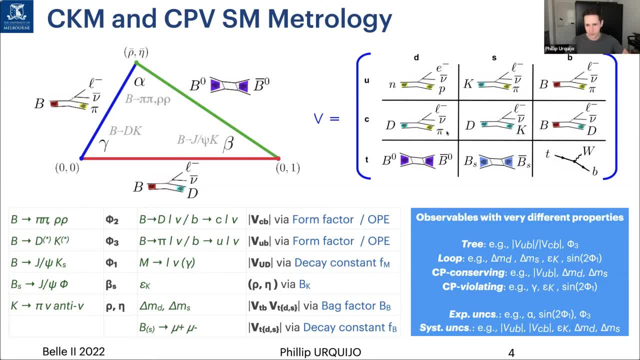 with semi-laptonic and leptonic transitions. These are the ones over here. from beta k's You can extract similar ones which are neutron and k under k. Putting all of this together, particularly measurement of the CP phases and the CKM matrix elements, allows us to. 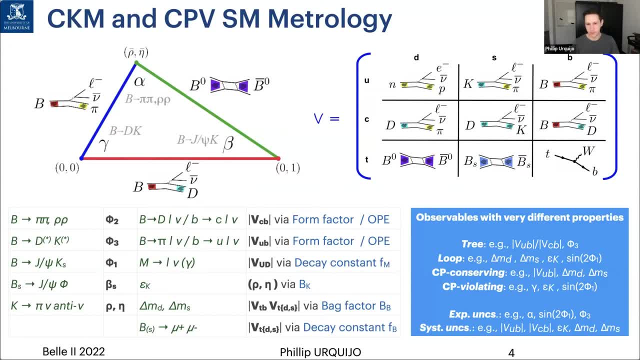 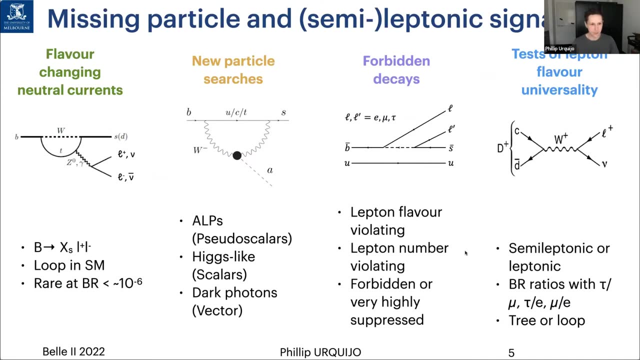 test for new phenomena. in different types of comparisons We can look at tree only versus loop only, CP conserving versus CP violating, to determine a potential pattern for new phenomena that can come through. The other type of physics that we like to do, particularly in beta k, is looking for missing. 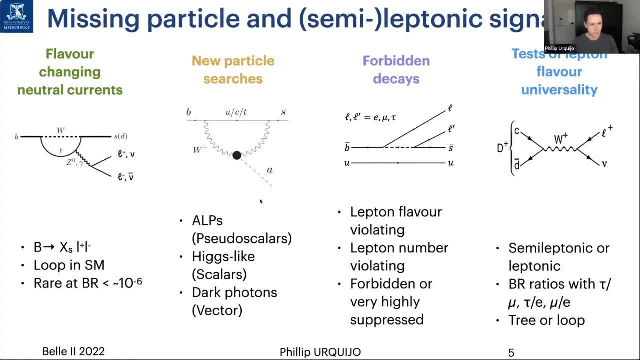 particle, leptonic and semi-laptonic signatures. On the first category we've got flavor changing neutral currents that can give rise to dilapton final states. A second one was associated to these feeble interactions and new particles that may disappear, So alps or Higgs-like scalars. 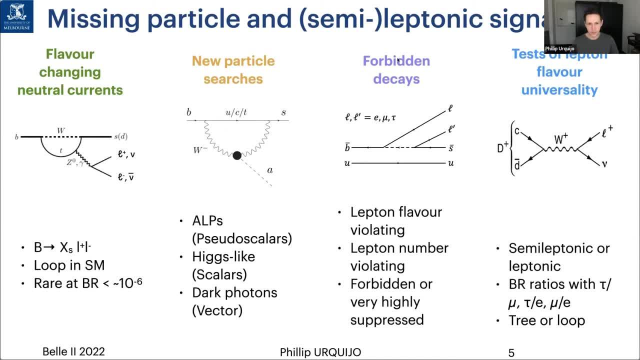 Or dark photons. This third one is on forbidden decays. Essentially, you break something like a lepton flavor number or lepton number, or it happens to be highly suppressed. And the last one is on leptonic decays, specifically tests of lepton flavor universality. 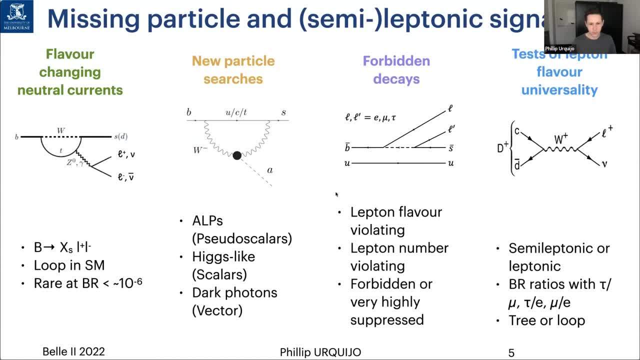 in this particular scenario. So those two major categories: one is CKM: precision tests and studies of CP violation and missing energy and leptonic signatures. The second category is leptonic decays, Two of the bigger themes for a B factory. Okay, so let's look at the collision environment now. 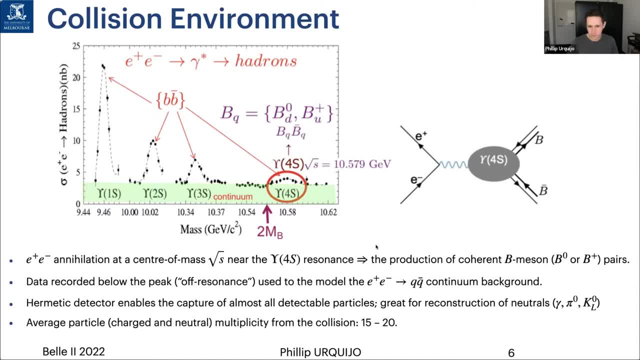 Most of our data is collected near the epsilon 4s. This allows us to produce coherent B meson pairs. But we also take a little bit of data that's just below, around about 60 MeV below, to collect background. This is very important to be able to suppress, to understand what. 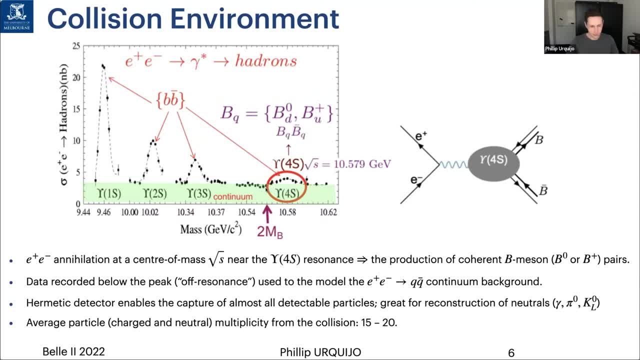 that background looks like to suppress it and to subtract it if need be. The cross-section for a continuum core production is around about 4 times that of B production, So that's why that's so important. The environment, because particles are produced near rest and we want to be able. 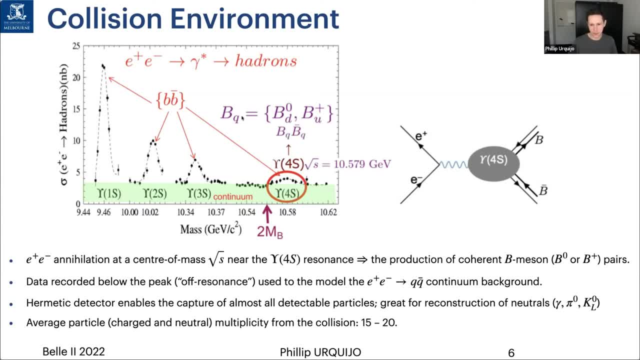 to reconstruct everything for doing a complete set of physics analyses. we want the detector to be hematic. We also want it to be very good at reconstructing neutrals such as gammas and pi zeros. We also need to find as many charge particles as possible. We want the tracking to be as efficient. 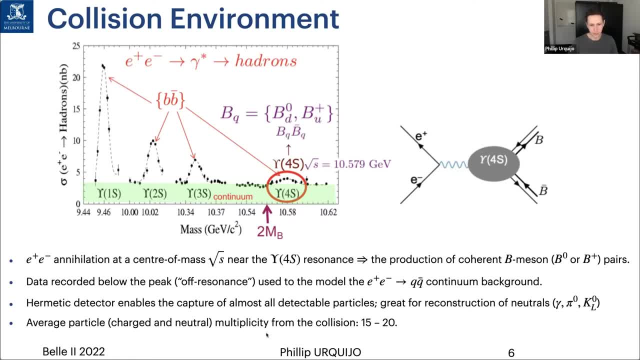 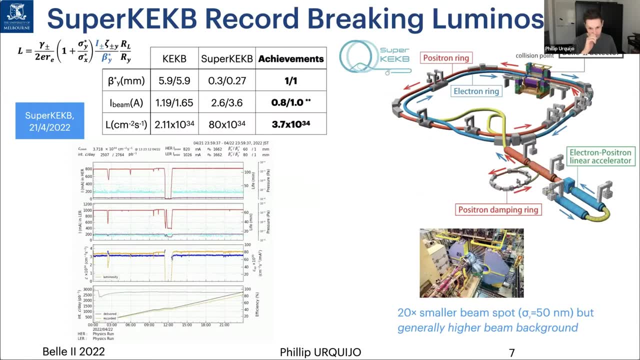 to very low momenta. that means that we need to pick up up to, you know, 15 to 20 tracks, neutrals in an event. well, um, of course, uh, superkick b has been operating and breaking luminosity records. uh, this is a picture from the 21st of april, so a couple of weeks ago. you can see uh pretty much. 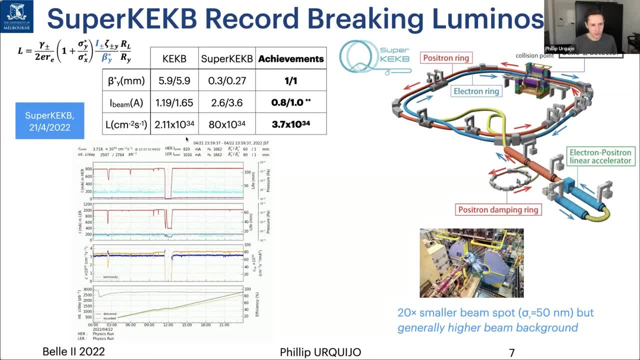 a record-breaking day of a peak luminosity of 3.7 by 10 to the 34 per centimeter squared per second. that's, that's what's been achieved, and here is is well, here, ballpark is one of roughly the uh, uh the target. this is already in excess of what was achieved at kick b and that's the. 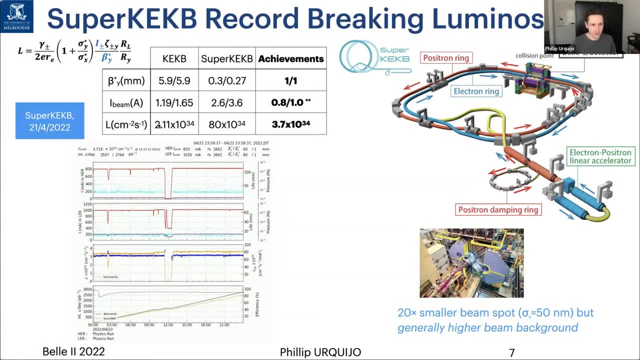 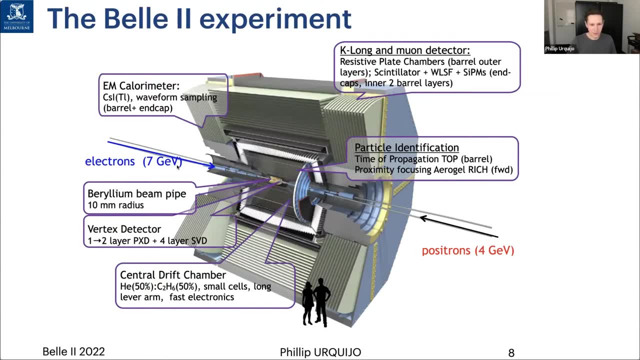 main comparison here. we're almost double that now, so that was the previous uh peak. as for the experiments, well, almost all of the experiments constructed, almost all of the experiment is there and has been there since the uh 2019 and operating uh. the exception is that this part of the vertex detector that's not quite there. 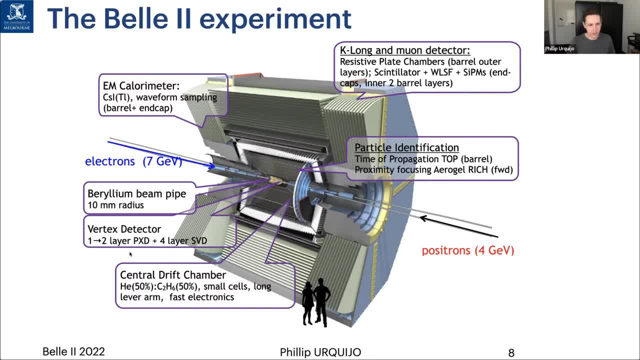 it's that currently operating is mostly a one layer pixel detector, uh, surrounded by four layer svd, and i'll come back to this. this is part of the upgrade program for the future. uh, outside of that, of course, we've got a drift chamber which allows us to measure track momenta. uh, that first one is: 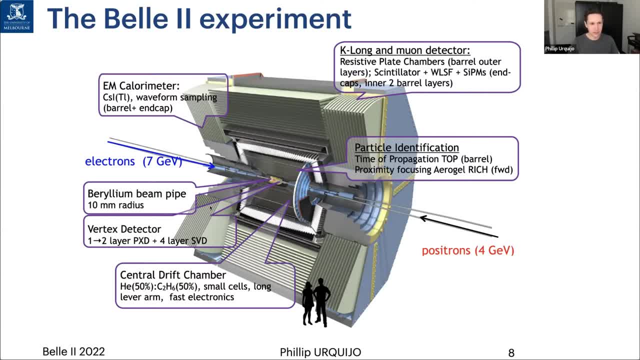 vertex detector because it reconstructs vertices um. next can comes the particle identification detectors that are primarily used for um separation of kaons and pions, but can also be used to separate out leptons. then there's the calorimeter, which is fantastic for neutrals, also very important for 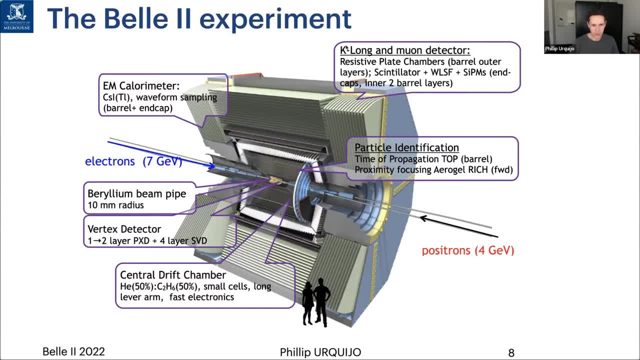 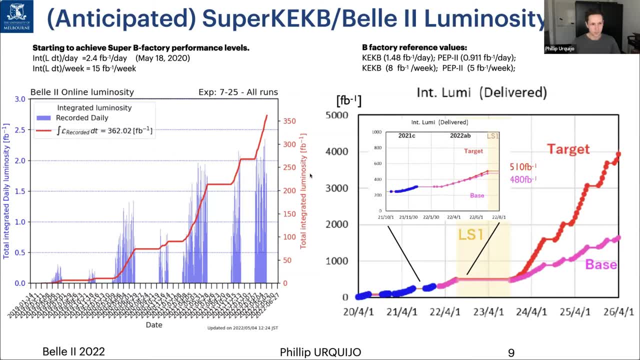 uh for electron identification, and then beyond that is the, the klm. this is outside the solenoid. so the data that's been collected from these collisions today has has grown to a level that's achieving uh. they're starting to achieve a lot of performance and they're starting to achieve super v factory performance, as i showed you. 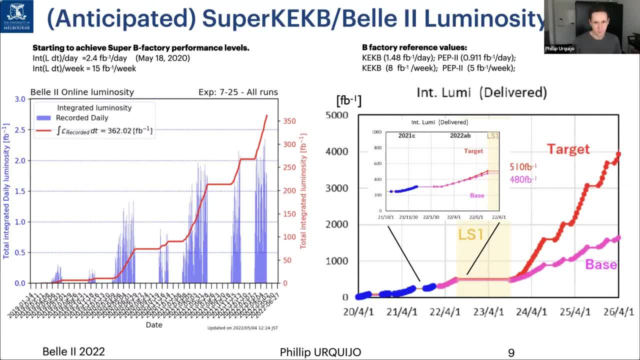 the the peak gloomy is almost double that now, uh, and the integrated data collected per day is up to around two and a half inverse temperature bonds. sorry about this typo here. um, that corresponds to about 15 inverse temperature bonds a week, and this, this you can see from 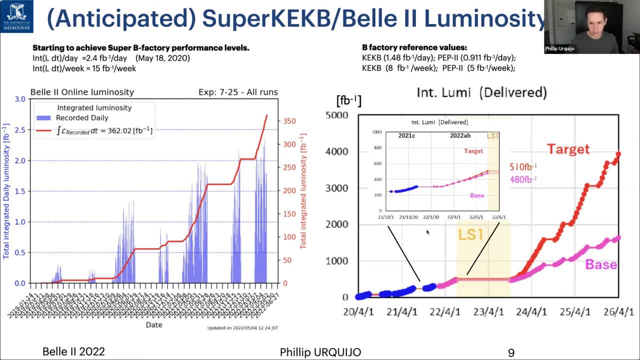 from the graph, the goals, though, as shown over here: um, we're coming up to a long shot shutdown period, um, and uh, so, uh, so we'll continue to take data for a bit longer and then we'll we we head into a shutdown period, um, before opening back up in a border a year's time. before continuing on, i'll come back. 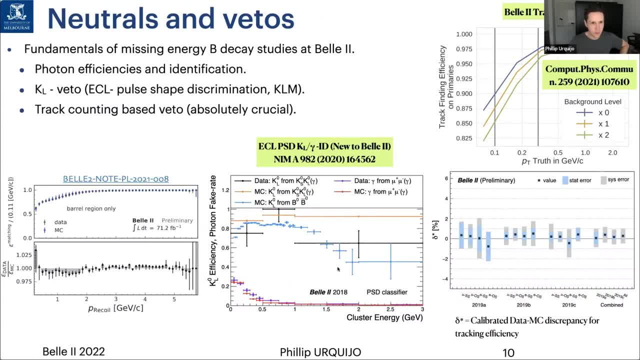 to what, what's going into these periods. so what about the performance of the detector? we need to know that it works as well, uh, at least as well as bell. uh, firstly, i'll talk about neutrals and vetoes. so here we've got photon efficiencies. uh, over here. 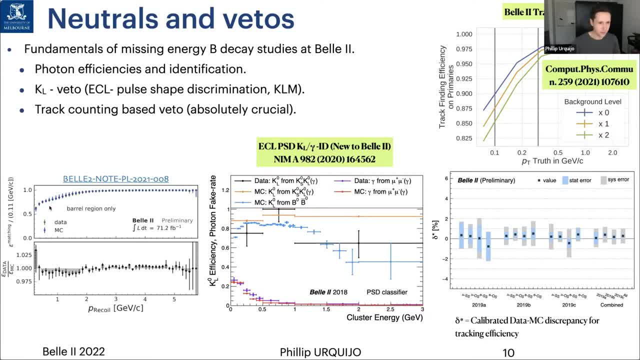 we can measure the photon efficiencies using uh tagged events and we we can see that the efficiencies in the data versus mc for these efficiencies, uh is very good. our particle identification for neutrals is also quite good. so we use this particle identification to separate out photons from from k longs, and you can see here: 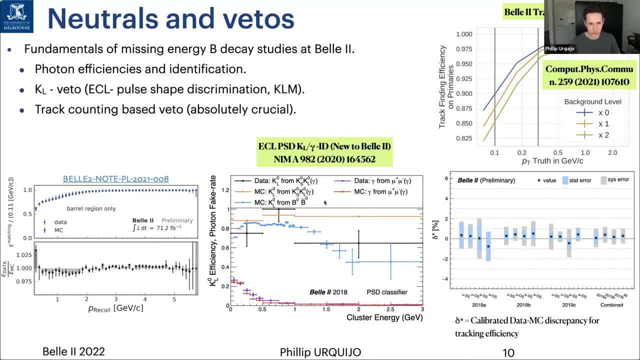 we can, we can. we can achieve that using uh, the calorimetry, uh alone, using pulse shape discrimination hand side. I've got recent results on track efficiencies down to low momenta. you can see that the track finding efficiencies are in excess of 90 percent. plus we can measure their systematic 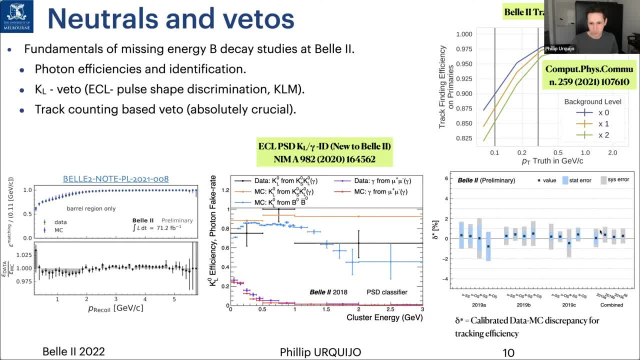 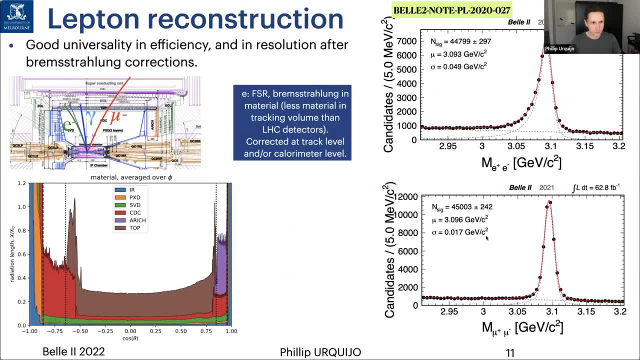 errors very well. this shows you that when we check data- mc agreement on our data, on our tracking- our Monte Carlo is working as expected. now. next comes lepton reconstruction. a lot of the channels that I talked about actually have a electron or muon in the final state, and it's very important to have. 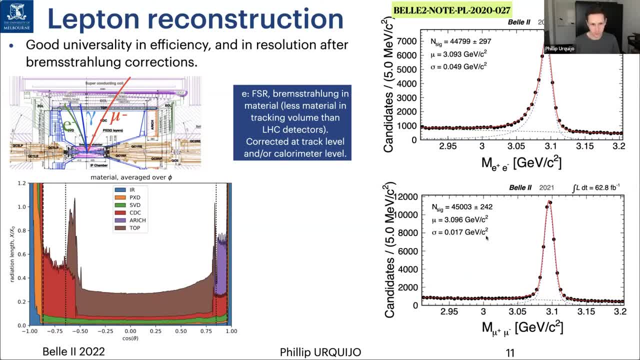 good universe. universality in the efficiency, if you can do it, so an experiment like bell 2 can do this. here I've got a collection of j psi events going to plus e minus and a collection going to mu plus, mu minus. you can see that one of them is a little bit broader than the other. 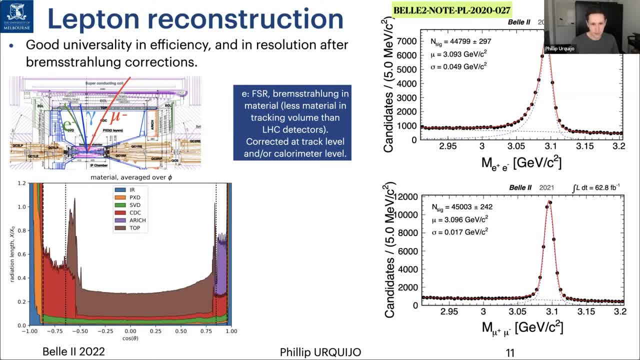 the electron loses energy via brems stradling in the material. that's due to the amount of material that's in in front of the detector. so in in bell 2, in front of the tracking volume, there's actually about 0.1 radiation length. this isn't so much and that's why this tail. 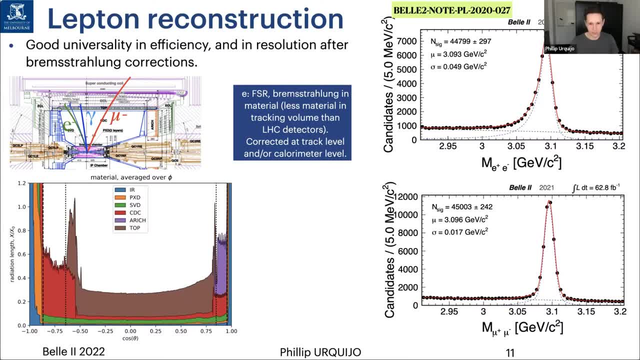 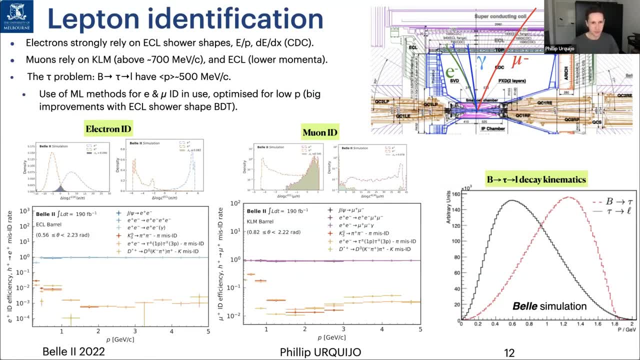 isn't particularly large, but in the case of LHC experiments it's significantly larger. okay, next comes lepton identification. so you've reconstructed it. can you tell the difference between an electron and a pion? so for electrons, we often use information that comes from the electron and the pion, so we can tell the difference between an electron and a pion. 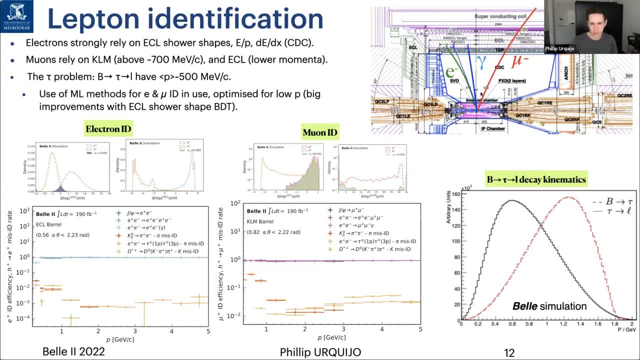 so for electrons we often use information that comes from the electron and the pion, from the calorimeter here, as well as information from ionization, energy loss through the drift chamber. this, this I've got pictured here for an electron and a pion. we can see: 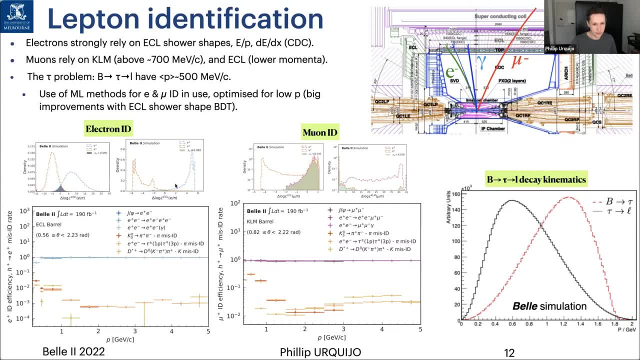 that their likelihoods are separated out quite well for the cdc and exceptionally well for the calorimeter. in the case of muons, we generally rely heavily on the muon detector, the klm muon detector, above around 700 mev that's enough to get past the 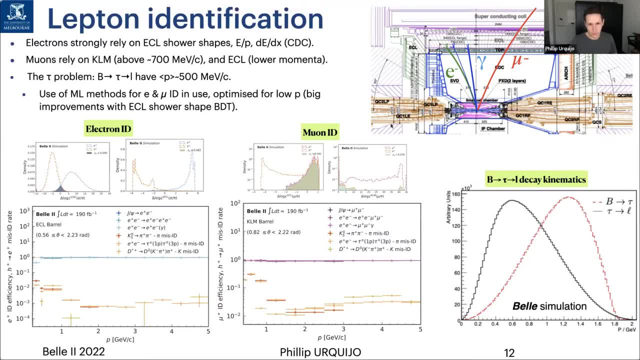 solenoid, and we can also use the calorimeter at the low end, and this actually shows you how we can. we can do so with the respective likelihoods for separation. then we throw them all into a machine learner and we get very good fake rates. and we get fake rates of order- one percent in the case of electrons at a 90 efficiency. 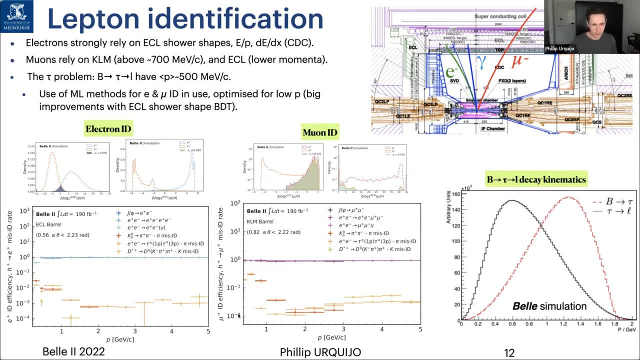 and a few percent. in the case of of muons are there a few percent, as you can see here. that's one of our goals is actually to measure at very low momentum, such that we can suppress background to measurements that contain taus, because they generally have low momentum leptons. 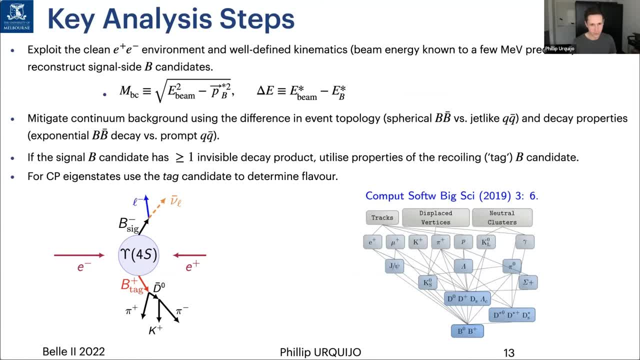 next we've got key analysis steps. so the environment- that the aplastic minus environment- gives us well-defined kinematics from the beam energies and we can measure these to a few few mev of precision. so we generally rely on beam energy constraint mass and beam energy difference parameters for background constraints. 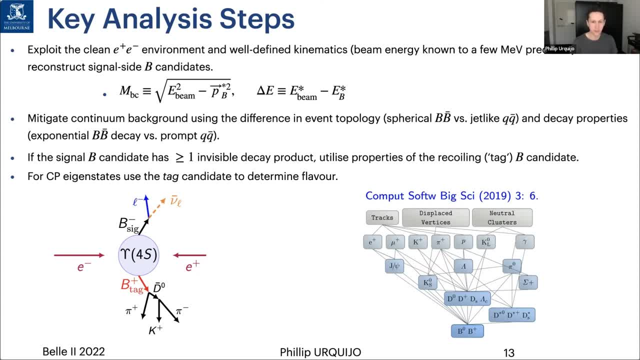 furthermore, we can mitigate a lot of the continuum background in our events using spherical versus jet-like topologies, so spherical for bees and jet-like for continuum. other tools that we can use are on tagging, so of course, we always produce bees in pairs like this, if you've got. 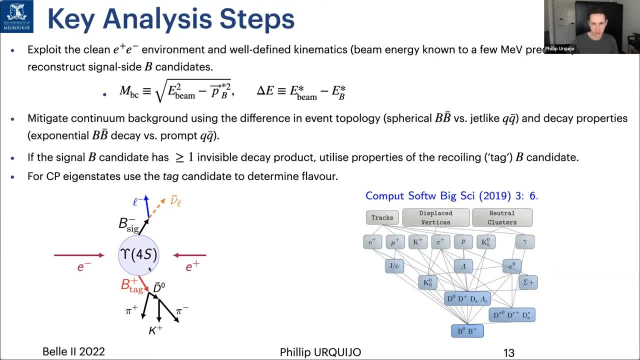 a signal side like this one with at least one invisible decay product, you can constrain the kinematics of that neutrino using the kinematics of the other side. so we do this often with techniques like fei, which does this complex set of full reconstruction of of. 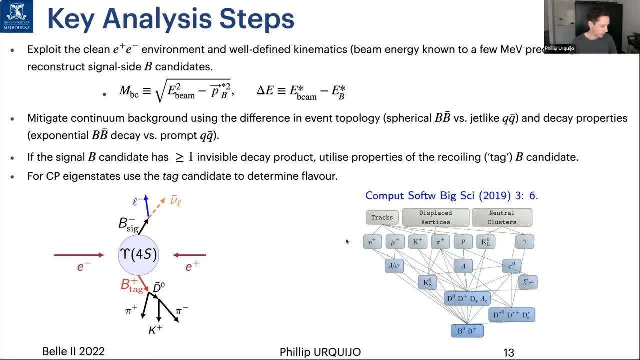 the tag side b. but we've also got um, a machine learned, complex algorithms that can determine flavor with very high efficiency. so instead of worrying about the full kinematics, you're just worried about the flavor of the b quark. you're just worried about the flavor of the b quark. 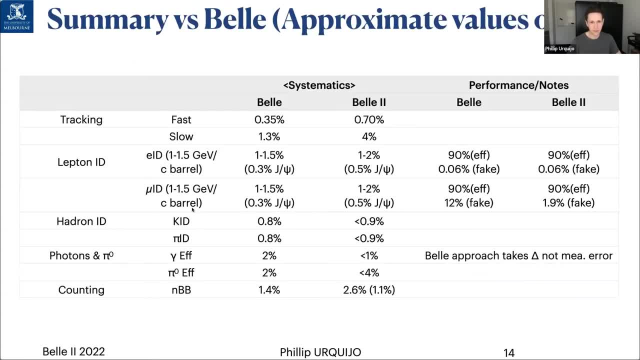 you can do that too. so to summarize- i won't go through this whole table- the current level of systematic errors and performance of bell 2 in the current data sets is now essentially reaching that of bell, except for a couple of places where, where we have slightly. 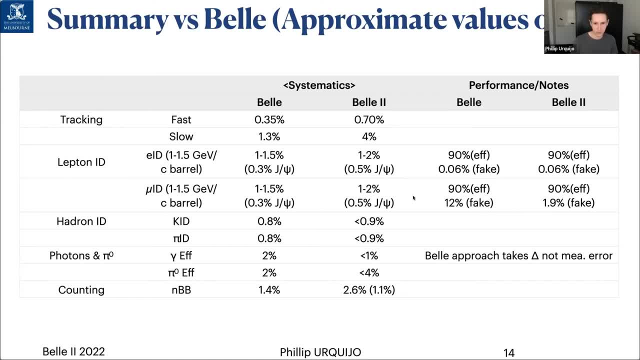 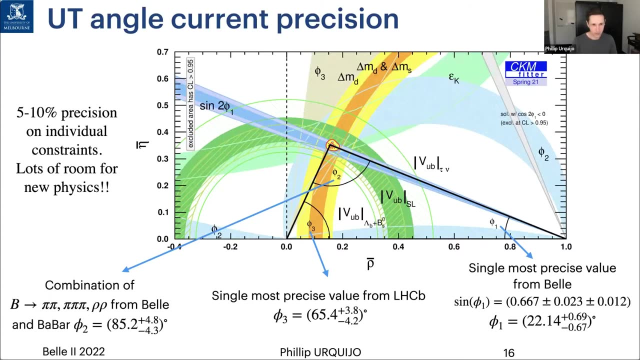 larger statistical errors, because our data set is just still growing at the moment. oh yeah, so i'm not going to go through all these. that's just a general remark that the performance now is as good or better than the predecessor. okay, so let's start looking at a few different areas. um the first one, i 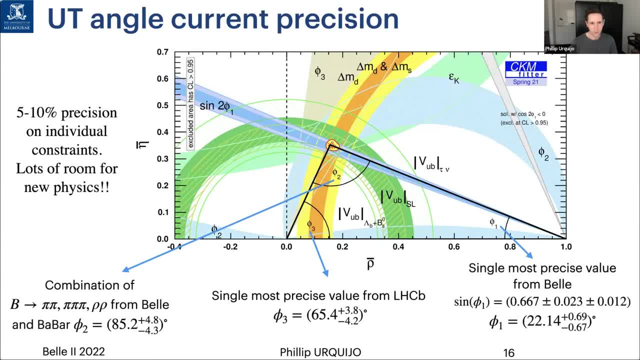 mentioned was on on cp violation. so the big goal right now is to improve the measurement of unitary triangle measurements. at the moment they're all good to around five to ten percent on individual constraints. that actually leaves a lot of room if you want to throw new physics. 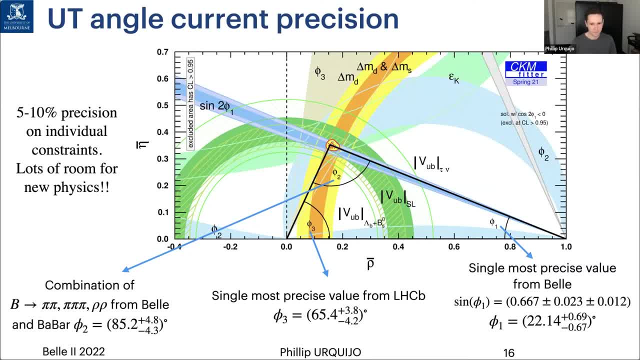 effects into the mixing hamiltonian, for example. so if you want to measure, if you want to compare new physics that enters via that loop and versus ones that don't, so the three main categories are, of course, measurements of phi one. the single most precise measurement at the moment comes from bell and in practice it's statistics limited. we can continue. 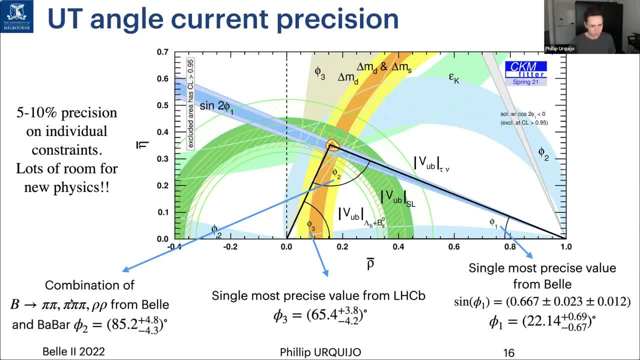 to improve this for quite some time. then, uh, phi two: this is dominated by bell and baba. its precision is six percent. there's a lot of room to improve here, and this will i'll get back to. and on phi three: at the moment, this is completely dominated, i have to say uh, from lhcb, which can achieve a. 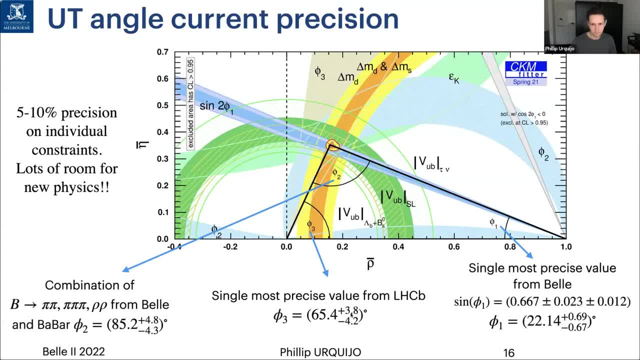 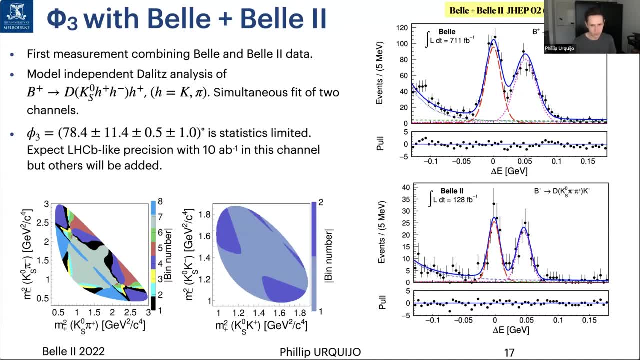 precision here, four degrees on the measurement of phi three. uh. however, having said that, um, there's now an effort to improve the statistical power of the of the b factory measurements and that, and so this effort was one where both bell and bell two data were combined. uh, you know, model independent. 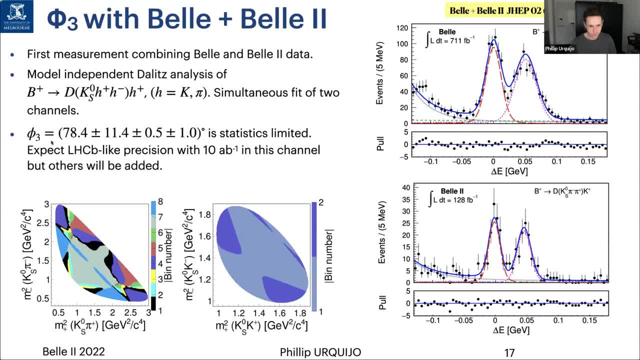 dialects analysis, uh, which was recently published, and you can see here that the precision is around 11 degrees. it's consistent with the previous result- and you essentially what you do is you measure uh, the b to d h, so k, short h h, uh h uh channels, uh, this is um the uh reconstruction. 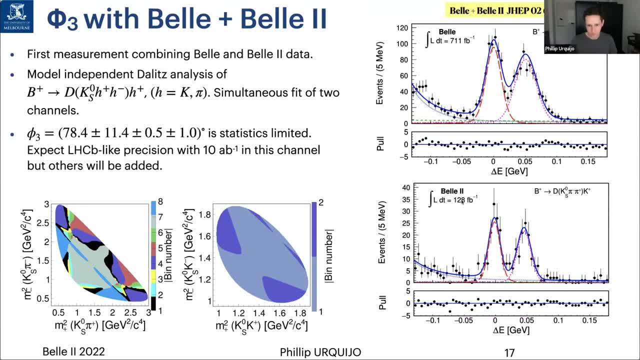 of the b to d h in the bell data set, so 711 inverse femtovans there and bell 2.. something you'll notice actually is that the separation between the two peaks here, that the pi on one on the right and k on one, so that's h equals k here and h equals pi here, is much better in the. 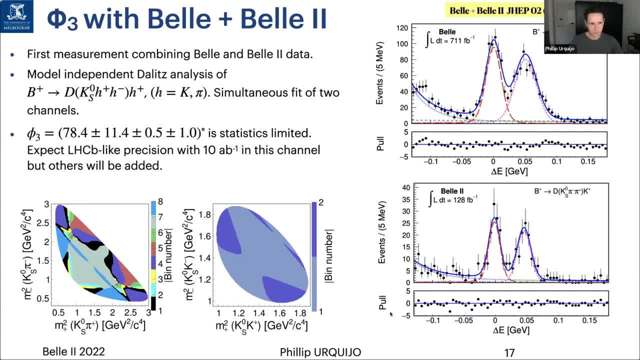 case of bell 2.. so just just a good example of how the statistical power of the data set has has improved. uh, we expect that it'll hit the current lhcb precision with around 10 inverse autobahns, but there's many channels to add here. 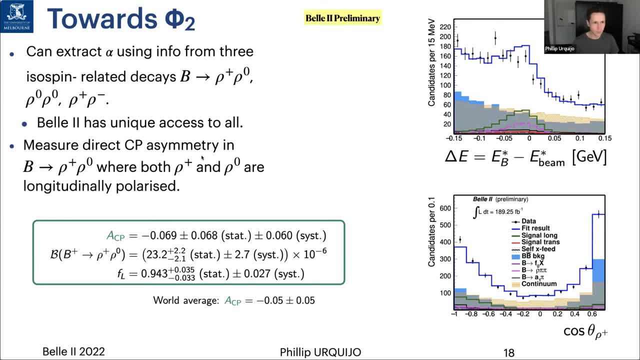 so the prospects might be better. on phi 2, you can extract this from three isospin related decays, for example. i mentioned pi pi and rho pi, but rho rho is an excellent method as well. so rho rho, rho plus, rho zero, the neutrals as well. this is an example: reconstruction of the channel rho plus. 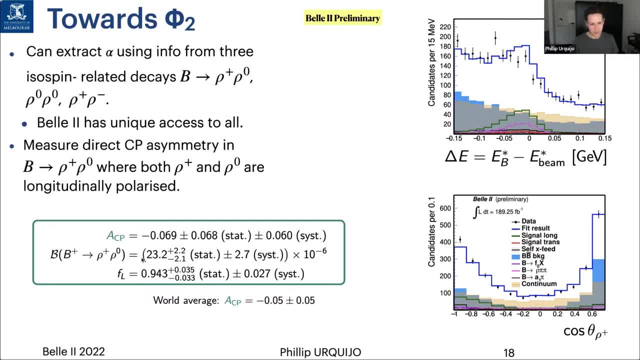 rho zero, so recharged v expresion of psi, v Karere and rho beta. so that brings us back to the main method where the direct cpo symmetry was measured. current level of precision is getting close to the world average. this is with 190 inverse vector bonds. 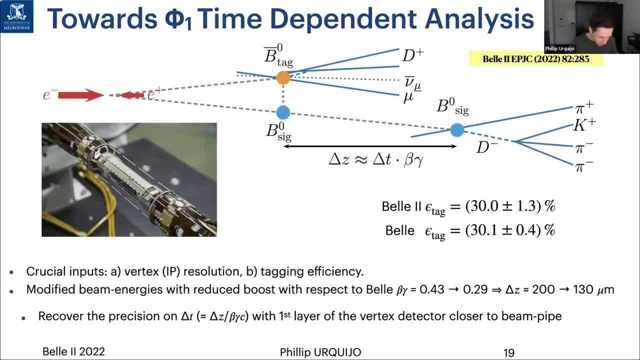 is measurement of Phi one. So Phi one requires that you measure the displacement between the tag side and the signal side B, Delta Z and you can relate that to Delta T, which goes into the time dependent mixing measurement. You also need to know what the flavor was for that tag side. 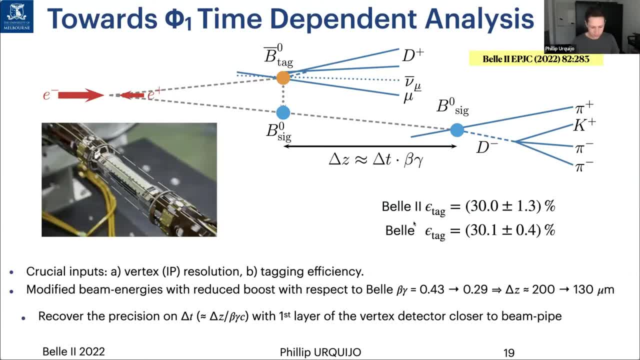 mentioned that before. At present the flavor tagging efficiency for Bell two is comparable to that of Bell. It's been measured and published earlier this year. Crucial inputs for this are the vertex resolution, So how well you actually measure these two positions and that tagging efficiency input. 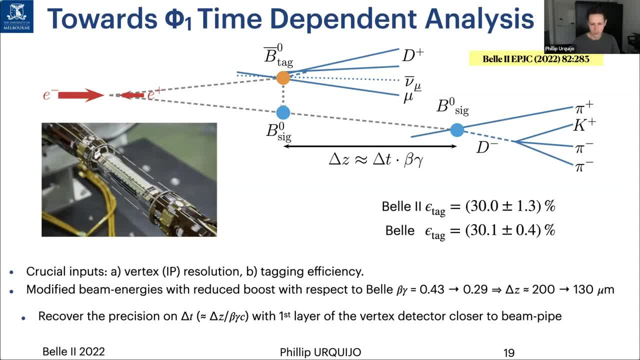 For Bell two, we actually had a reduced boost with respect to Bell And that means that you have to generally you have to compensate a lot for the reduced resolution. sorry for the reduced displacement, but this is done by having a closer vertex detector layer. 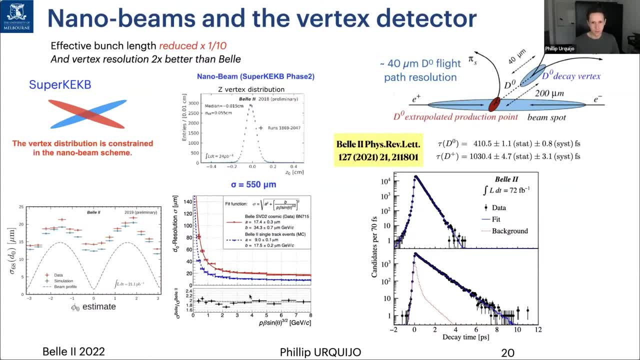 So something closer to the beam pipe. So I've got a picture of that up here. essentially, Yeah, I'll go through this one. So the solution for it was a combination of both nanobeams with the vertex detector. So firstly with nanobeams, 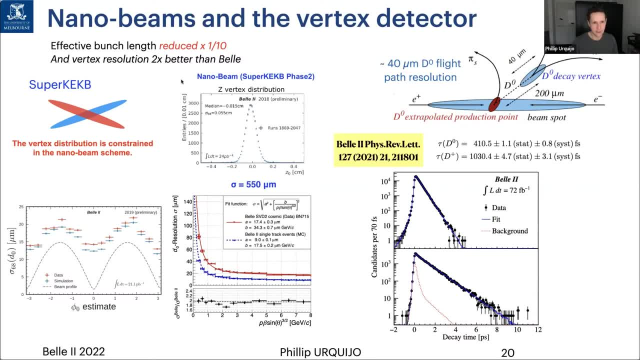 you get an effective bunch length. that's much smaller. That's about one 10th and the vertex resolution, but it's a lot smaller than the actual value. So that's the difference. And then the prediction for Bell, also reduced, is reduced by a factor of two. 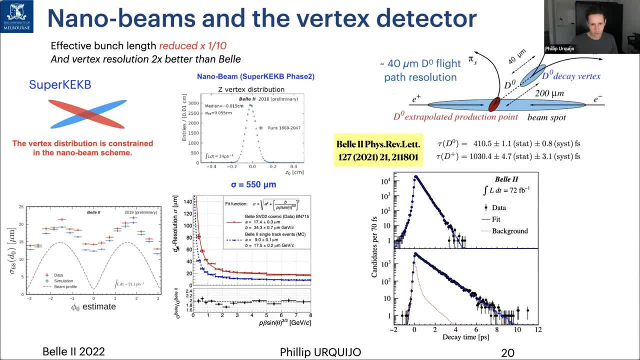 So the old Z-vertex distribution used to be around 10 times larger than this. This is 500 microns In the case of the D zero and the Z zero. so these impact parameter resolutions from Bell through to Bell two, these came down by a factor of two. 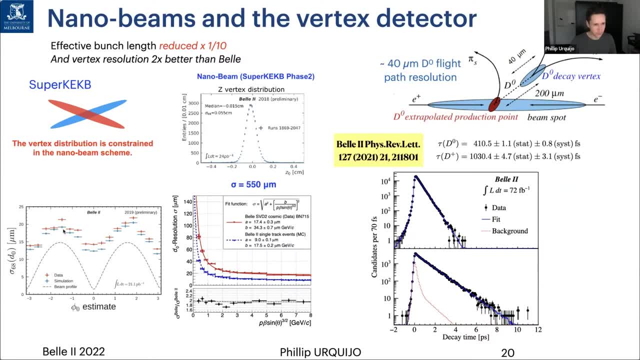 This is Monte Carlo and this is extracted directly from data: 12 to 20 microns. so this was measured in a something more than a demonstrator analysis, but I'll use it in that context, and that's the measurement of the charm: lifetimes. so the charm. 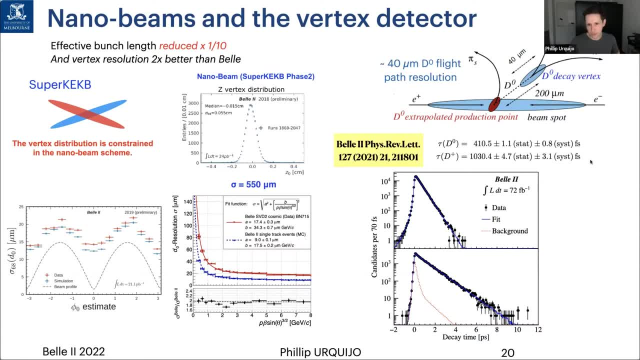 lifetimes. d and d plus were extracted. essentially, you determine the production point from the collision kinematics and measure the displacement so that flight path, and that flight path can be measured to a resolution, in this case, of around 40 microns. that gives you world-best measurements. 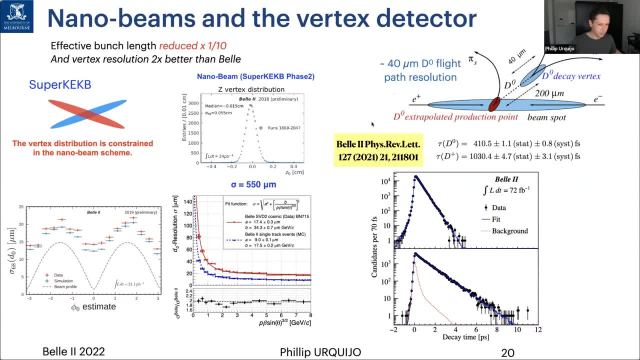 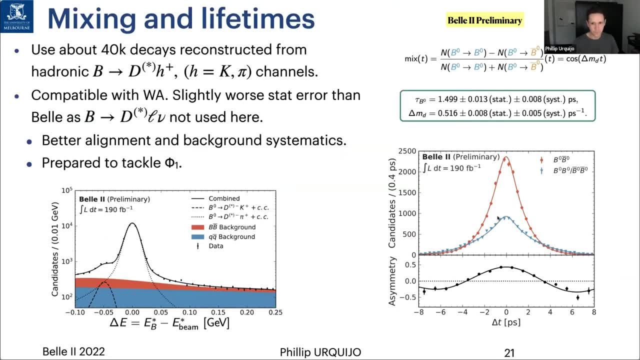 of the charm lifetime. so this is an excellent example that time-dependent cp violation can be performed, but on the way, measuring these at two prl level. okay, so that brings me on to the next bit, which is actual measurement of mixing in lifetimes. around 40 000 events were reconstructed. 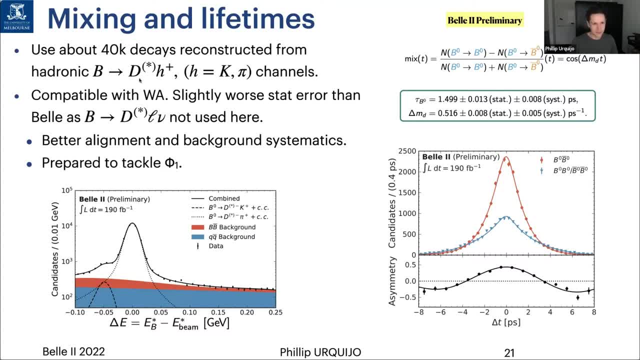 in d star and d, eight d star and d d plus a hadron where that was a k or a pion, and you can see this reconstructed in delta e, as this is the typical distribution you use for the extraction. so this is the d pi component, this is a dk component, and then you measure the mixing parameter delta md. 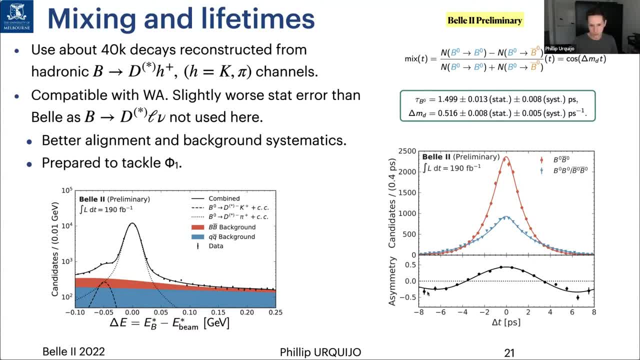 from a time dependent measurement of mixing and that gives you an asymmetry, and from the amplitude- sorry, from the period of that uh, asymmetry, oscillation. you pull out the delta md. this is comparable to previous results, uh, but the, the precision isn't quite as good as the, the best done by bell, and that's. 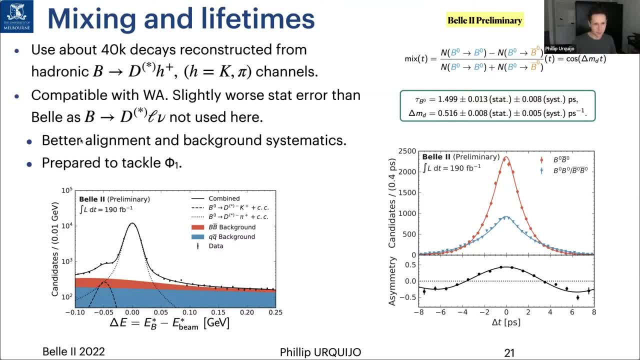 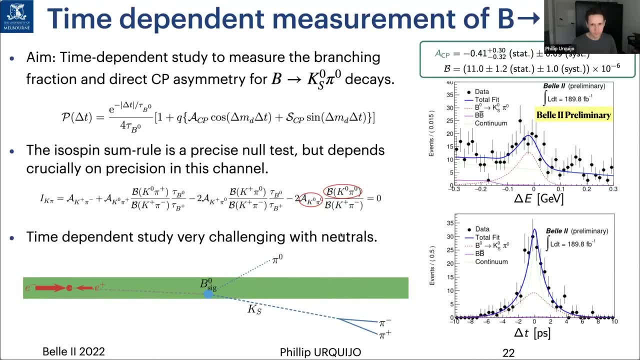 probably due to: we'll just need to add the channel that was used in that previous analysis. anyway. um, the systematics are much lower and we're ready to tackle phi one. okay, okay, on time dependent um time dependent measurements beyond ck metrology. uh, we look at. 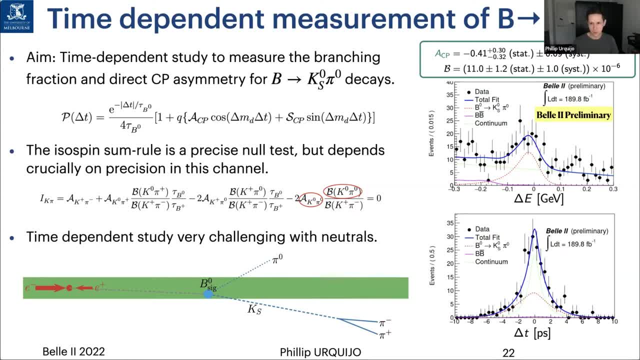 channels like k short pi zero. this one we look at because it proceeds via a gluonic penguin diagram and this means that it's potentially sensitive to uh, to new physics, in a way that other processes, like jsi k short tree level ones, are not as sensitive. 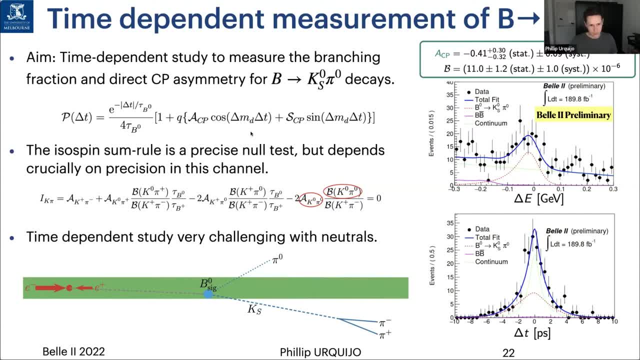 so the idea is that you can measure the time dependent, sorry, you can measure the amplitude of the cosine and the sine terms in the time dependent cpa symmetry, these, these, these are useful potentially in a precise determination of the isospin sum rule test. essentially, this relation here cancels out uncertainties due to. 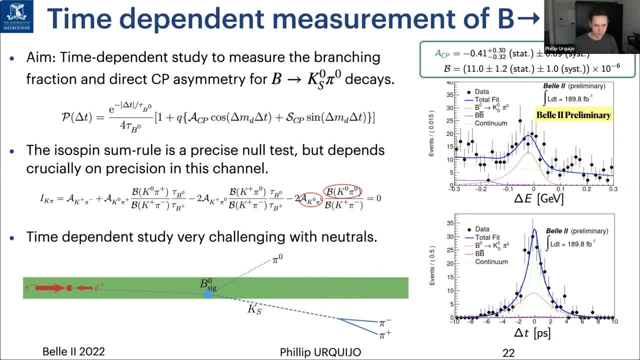 uh qcd related theoretical uncertainties. that gives you a precise null test of zero, but it critically relies on the import of the uh cosine amplitude term and the branching fraction of the neutral modes. this is the least well determined, so this is actually extracted from a time dependent analysis where you could simultaneously fit this in this. 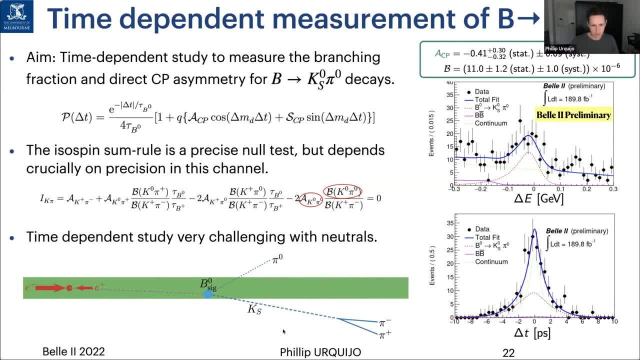 to k short by zero. it's very experimentally challenging because uh pi zero doesn't give you a good vertex And this is a long-lived particle, so it's challenging. In any case, Bell 2 pulled out a preliminary result on this. 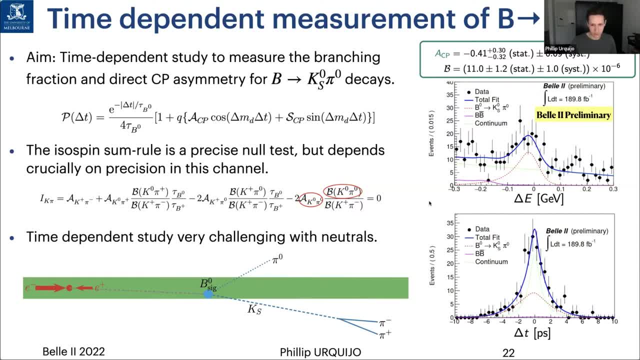 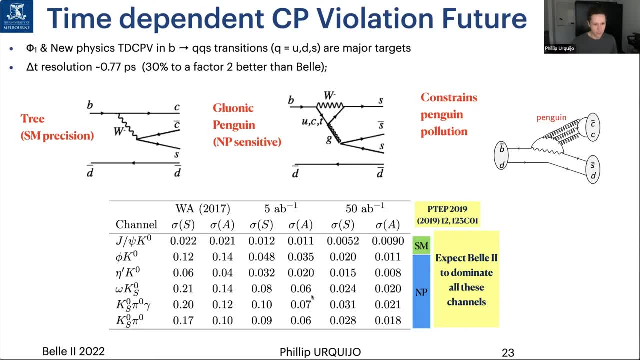 and this will soon become something quite competitive and useful for this kind of test. This is a really good one for new physics. So what about the future? That was one such measurement, So obviously phi one is very important, but so is time-dependent CP violation in beta QQS. 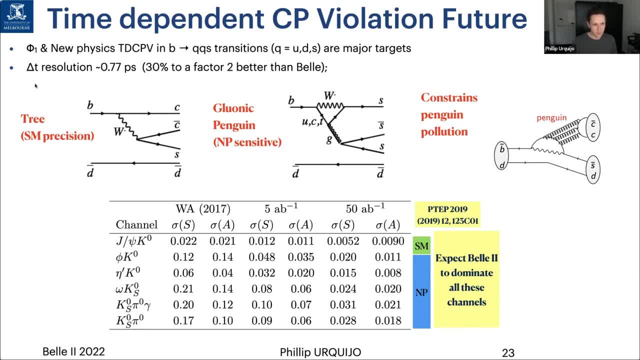 of different quark types. The delta T resolution is very good, so we're definitely gonna get better systematics And there are several categories that we'll be looking for. I mentioned tree, I mentioned gluonic penguins, and these are the two main categories. 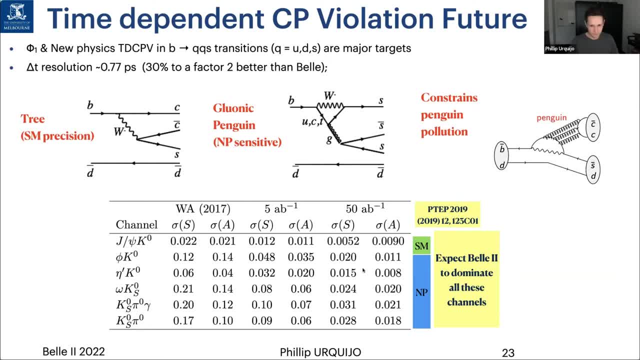 There are others that are important for systematic errors. So in the future we'll expect Bell 2 to dominate a lot of the channels that I've got listed here, and for the precision to continually improve and be almost entirely statistics-limited for almost all of these. 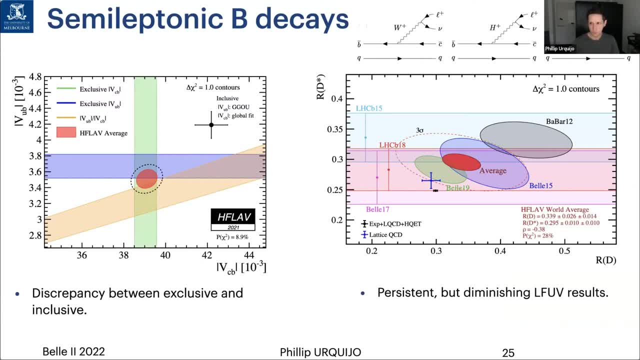 Okay, I'll get onto something that's maybe a lot more popular these days, in a sense, and that's anomalies in the form of semileptonic and dileptonic anomalies. All right, the one on the left is one that's been persistent. 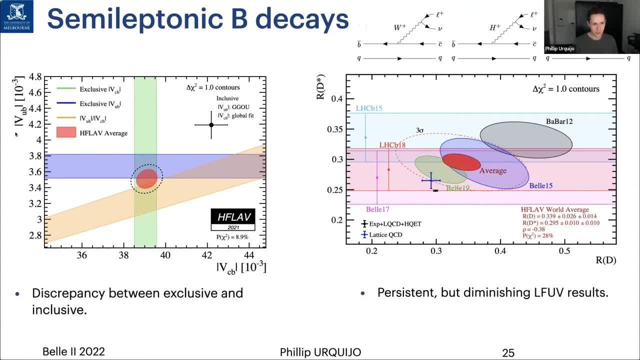 for really quite a long time and it's associated to the extractions of the CK matrix elements VUG. The top right dot here is the extraction via inclusive methods and the fit here, but the bands here are via exclusive methods, The ones that I would compare to directly. 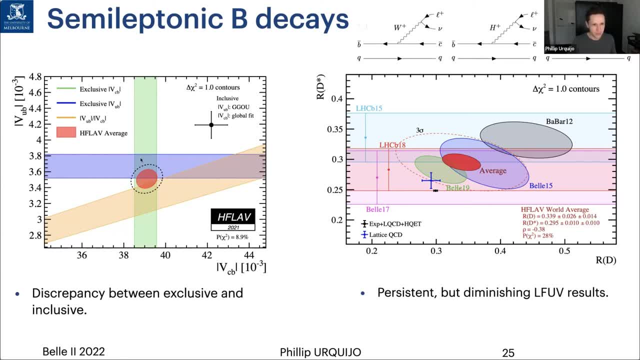 would be the blue and the green bands around this point. Orange is independent result taken from mostly baryonic inputs from LHCB In any way. I think it's a very good example of that. I think it's a very good example of that. 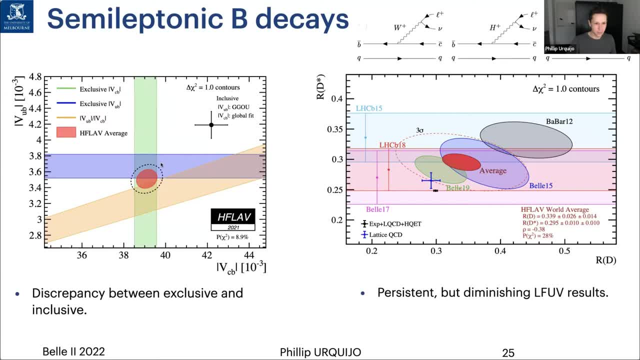 So, in any case, there's actually really a large difference between the extractions of these parameters and it's of order of three sigma. It's an open question. I'll get to what the current status is a little bit more later. 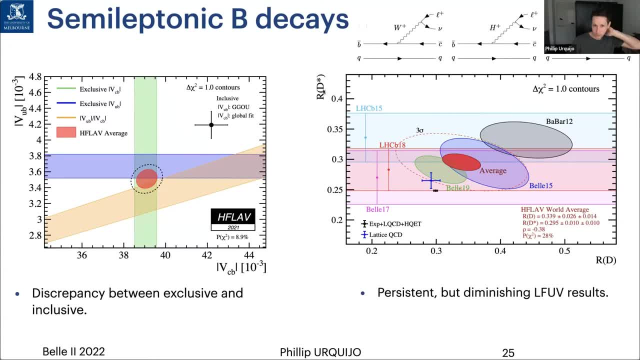 On the right-hand side. we've got our test of LHCB, so our ratio of D star tau nu over light lepton channels. And of course we do this not because we wanna measure anything fundamental. we wanna search for charge, Higgs or say HG. We wanna do this because we wanna measure anything fundamental. we wanna search for charge Hg or say Hg or say Hg or something like that. we wanna do this because we wanna measure anything fundamental. we wanna search for charge Hg or say Hg or something like that. 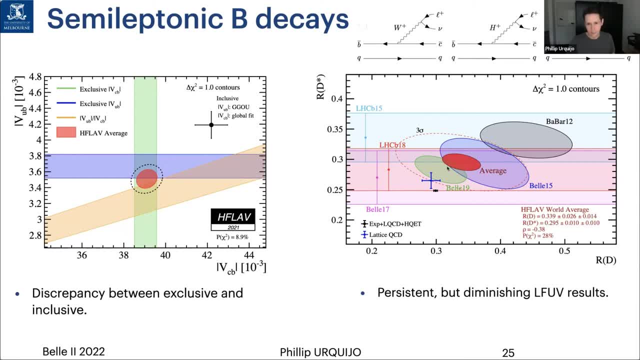 electric walk. the current status of this is that the world average in red is uh off the the theoretical prediction this being the more common one to take by more than three sigma. i should note that if you base your prediction purely on lattice qcd, it's a couple of sigma away. this is uh maybe a detail. 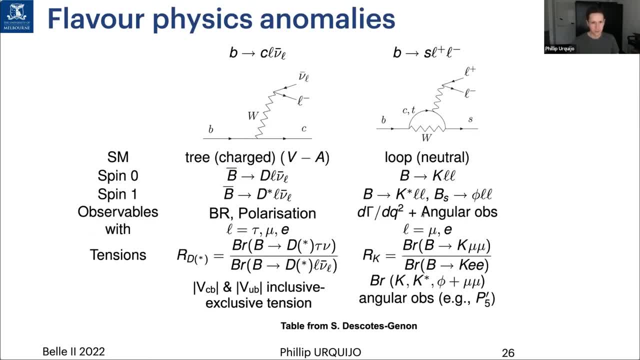 what you under 900, Democrat or higher, could be used is to estimate the 중요acy to take you. so now, this is an example of a multivariate. yourself here just to talk about the necessity of instФ". So this is. These are loop processes, similar types of observables. 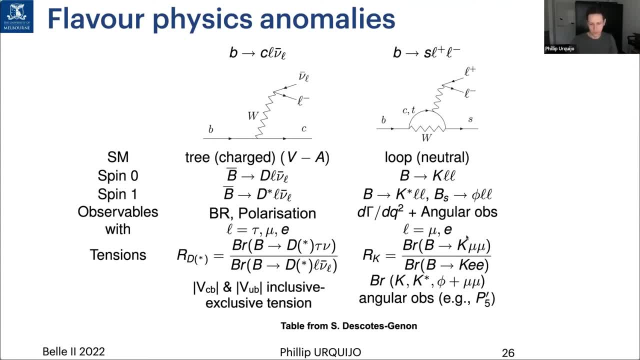 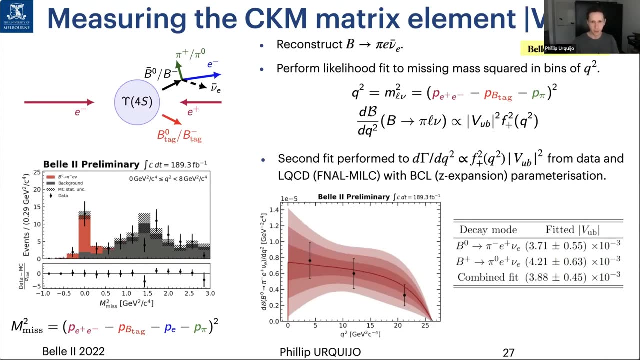 branching fractions angular observables, And we've got also discrepancies, but in this case in the ratios of mu versus E and in branching fractions. I'll come back to this one after I go through these. So in more recently, Abelto is providing input on the VUB. 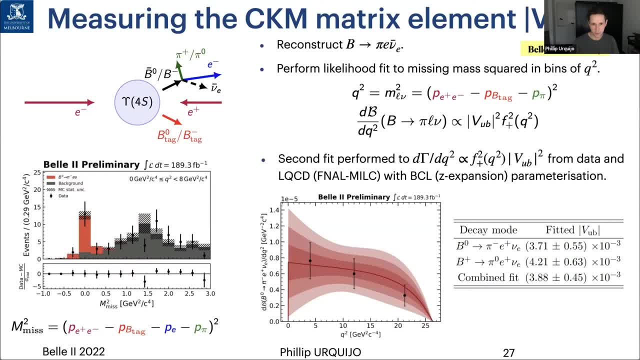 inclusive exclusive puzzle by improving the measurements of VUB. Here we use that tag method in beta, pi e, nu and perform a likelihood fit to the missing mass squared distribution. So essentially that's your initial collision, minus the tag, minus the pi on yep and minus the electron. 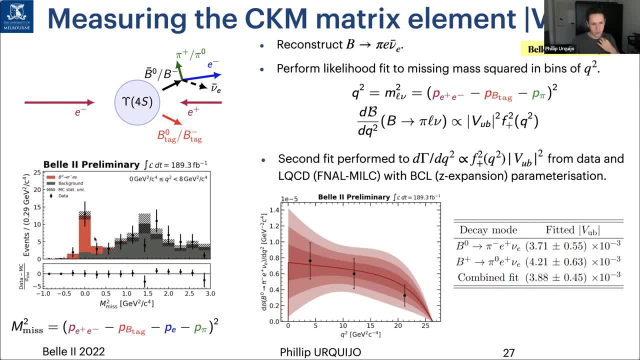 That gives you the missing mass and it peaks for the signal and it's actually pretty clean. However, because of the tag, the efficiency is low and you can see in this particular channel only about 15 events in this region. So we then fit this with lattice QCD information. 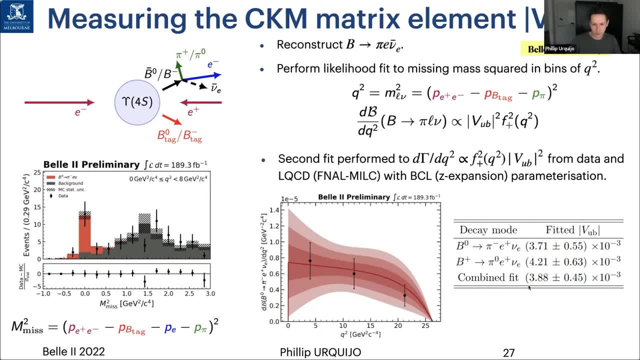 and pull out a value of VUB And we get a number of about 3.9 by plus minus 0.45.. So it's just over 10% precision already, with a fraction of the Bell dataset, But, yeah, all of the available Bell too at that time. 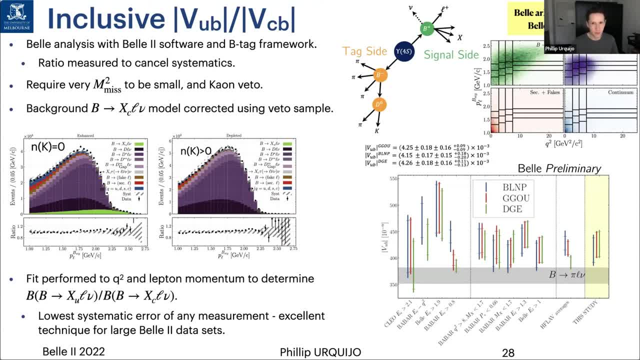 We expect that to continually improve with more data. of course, This is not a Bell two result. it's a Bell one, but it was just made public about two weeks ago And this is a measurement of VUB on VCB And it's something I'll point out. 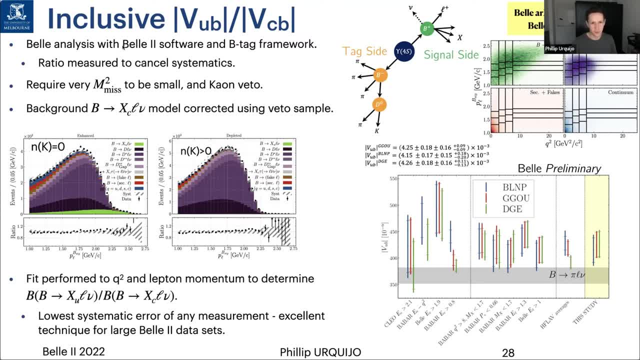 cause. my student did it. So it's a Bell analysis with Bell two software and the B tag framework, And the idea here was to measure the ratio, to cancel out a lot of experimental systematic errors, And we determine the background here using a data driven. 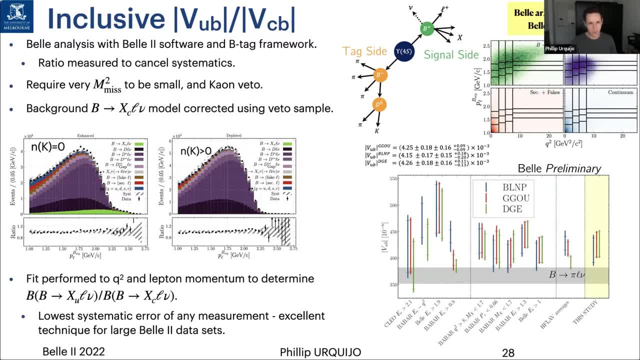 method, from a veto system, From a veto sample. So that's where you have a non-zero number of K-ons, which indicates that it's a background, from a cascade of a B to a charm, to a strange cork. You can see, here the signal component is excess. 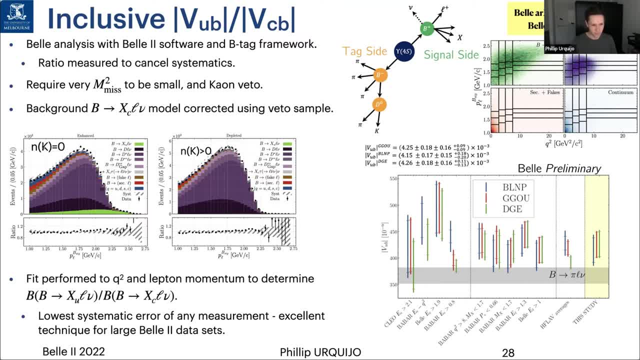 is clear in the category with no K-ons. So using a data driven approach to correct the spectrum where you can see there's a discrepancy. we then fit to Q squared and lepton momentum and determine the ratio. We don't have theoretical predictions for the extraction. 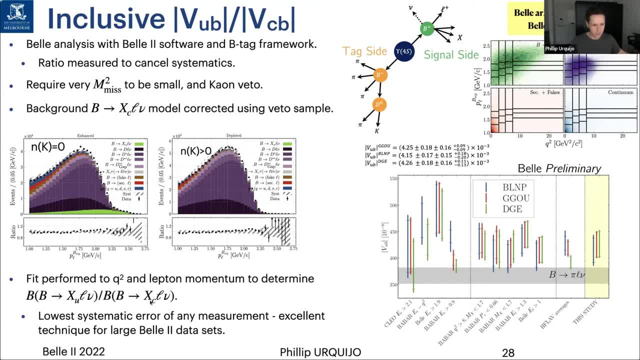 of VUB on VCB from that ratio yet. but we can multiply through by that branching fraction at the moment and get some values of VUB. So comparing that to that beta pile, new result: well, not that one, the world average. 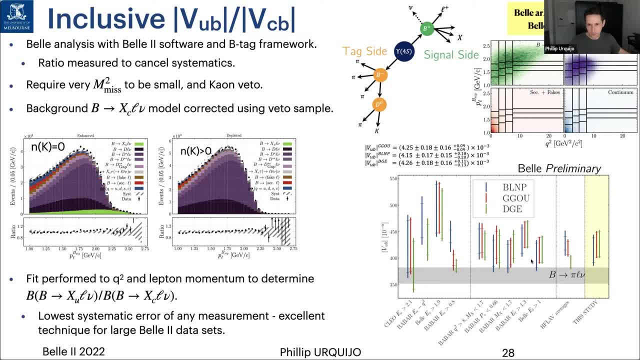 the new study is here, and the one that was published in the past year from Bell using a complimentary techniques is almost the same central value, but with low statistical overlap. So you can see that now we've brought down the tension with respect to the previous page by quite a bit. 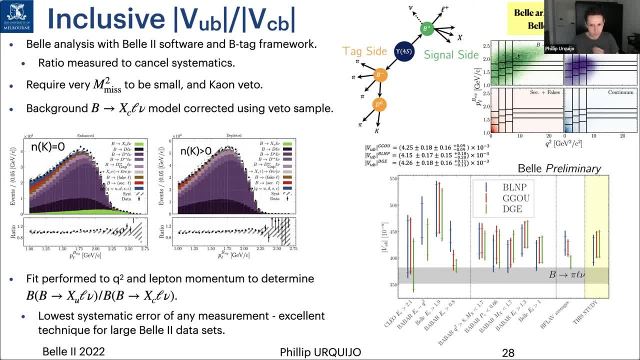 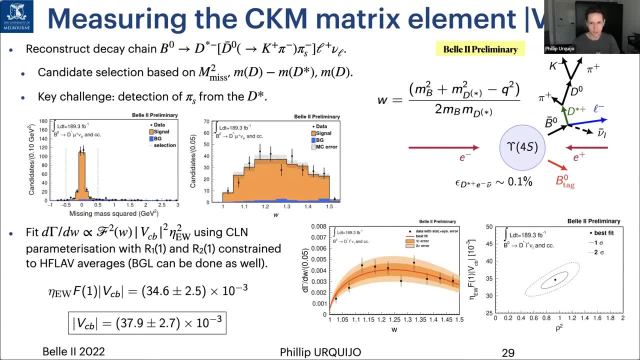 I think we're closing in on that gap. Bell two, I think, is gonna have to finally resolve it there. Okay, Then for the heavy to heavy, we've got VCB. We usually reconstruct this in a semi-leptonic channel. 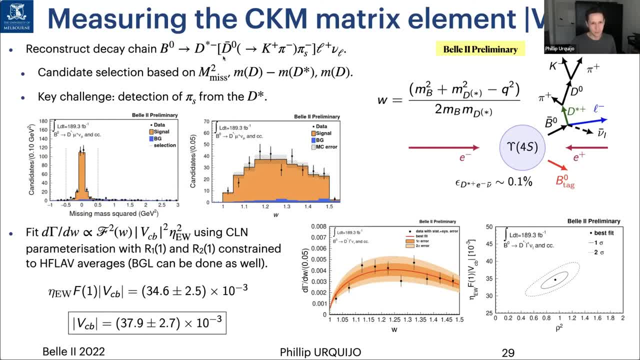 like a D star, L, new, And then measure the W distribution. This is a hadronic recoil distribution And the reason why we do that is because hadronic recoil is important for the theoretical calculation. When you wanna theoretically describe a transition like this: 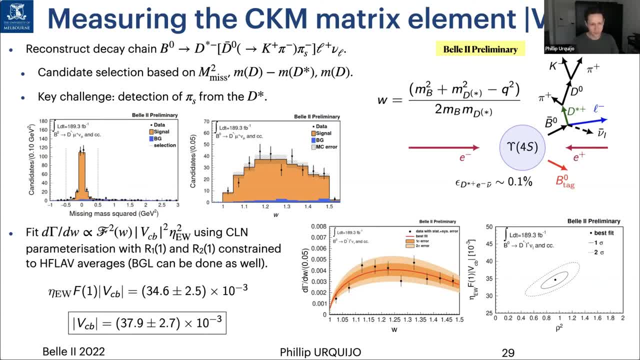 you relate the decay differential to a form factor and then VCB squared, You can precisely calculate that form factor If the initial meson and the final state meson have fully overlapping wave functions. So that means that the D star is at rest in the B frame. 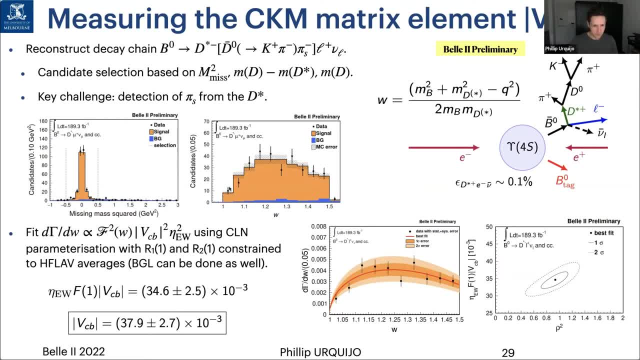 So what we really want to get is the kind of overlap down here at W equals one. That's, the information we really want is down at this point, Actually. so that means that the key challenge is detection of slow pions, because this corresponds to very slow pions. 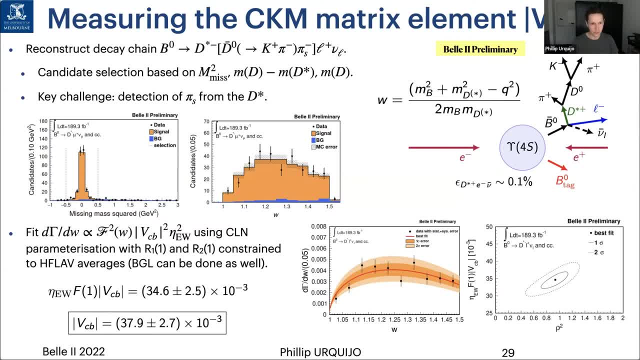 Experimentally. that's much better in Bell two, So we expect the systematics to be significantly better than in previous. In any case, this measurement was performed and we pull out an exclusive value of VCB, which is on the way to high precision and not there yet. 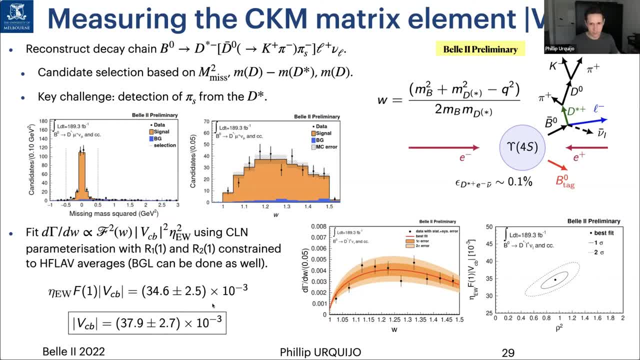 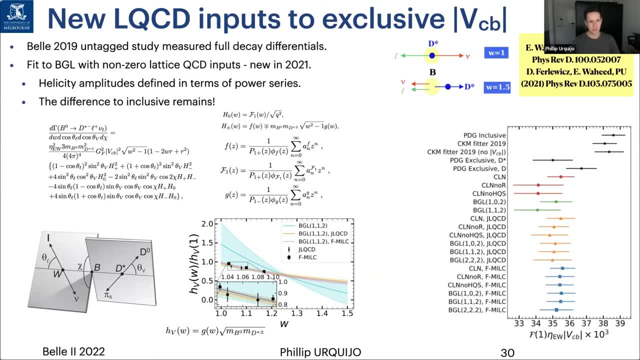 but highly statistics limited at this point. On top of this there's been a lot of new import from lattice QCD, So I mentioned that. you want to know, if you want to calculate, compare your measurement at hydronic recoil of zero. 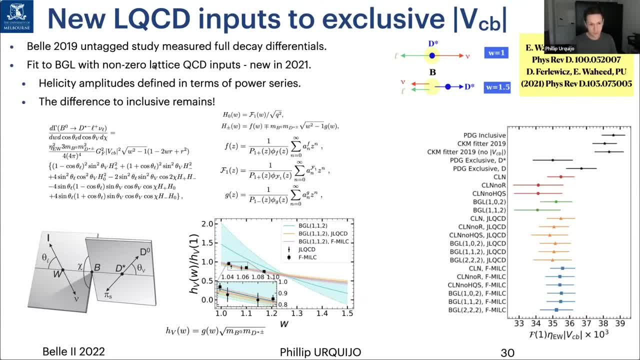 So this particular configuration. There's now been non-zero lattice QCD inputs that were brought into the field last year and it kind of transforms how we do these measurements. So Bell actually published some untagged data for this and you can relate. 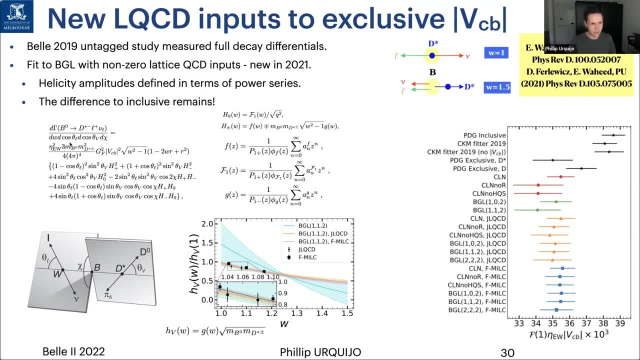 essentially you can measure the decay differentials in three different angles. So you can see that the and W- this is related to a theoretical expression in terms of elicity amplitudes, And then we can write out those elicity amplitudes as a, as an expansion down here. What we can also do is extract where we can take predictions for elicity terms- Sorry, the form factor terms- from lattice and constrain them heavily as well as fit to the Bell data. 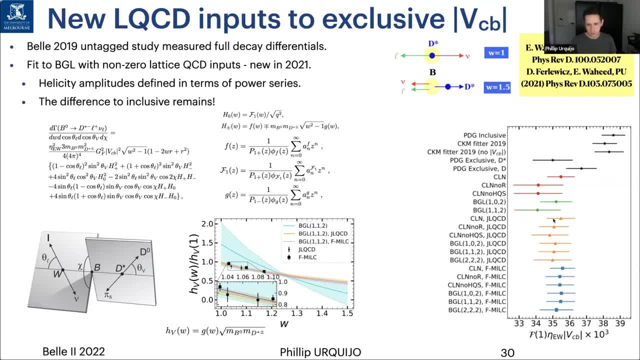 And what we found was that. and what we found was that, whether or not you included that information, it turned out that the results were incredibly consistent, just that the uncertainties had come down. So, essentially, without much lattice information, we get a value that's similar to the black line here. 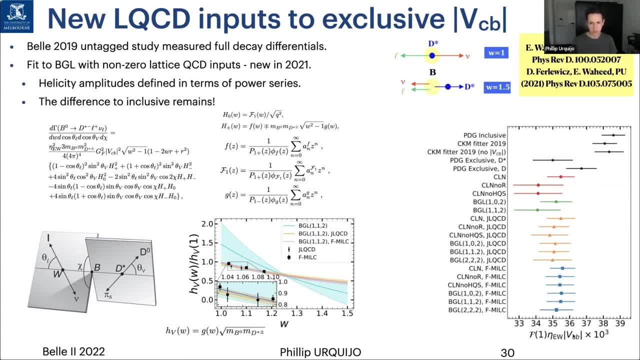 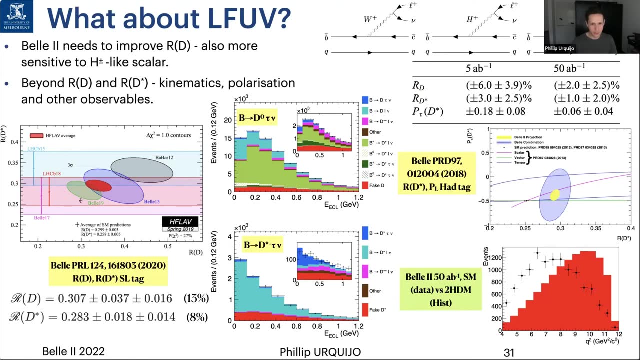 and then through different other configurations, we see very little variation across the fit results. It was very interesting, but it says that the puzzle on the VCB side is still open. Now, I didn't mention LFUV yet, So what about that? 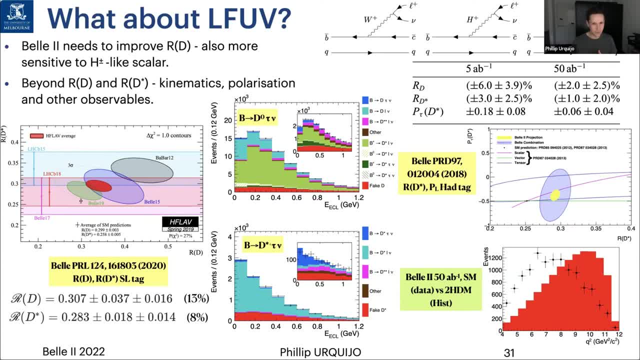 There aren't any measurements out from BEL2 at the moment, So let me just talk about the prospects for these Here. I showed you this figure before. The single most precise measurement came from BEL in 2019, using BEL2 data analysis software. 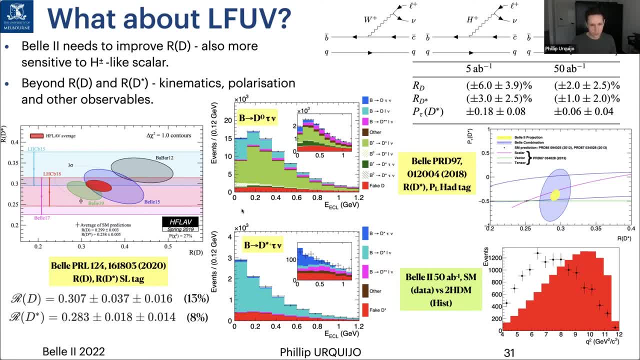 There was a simultaneous measurement of beta D tau nu and D star tau nu, And that's how this could be extracted here, And the approach was to use a semi-lactonic B tag on the tag side. In the future, of course, with more data. 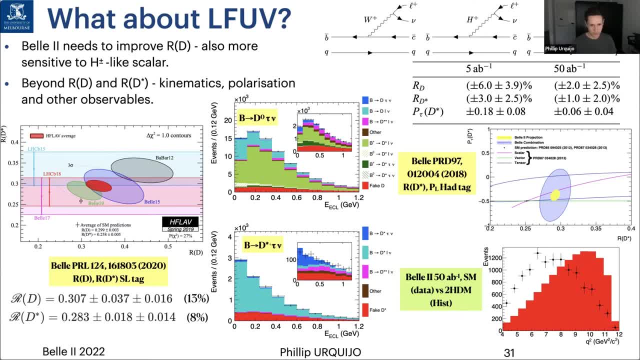 you'll do this measurement again, of course with more data. you'll do hydronic tag. You look at different decay channels of the tau lepton. you look at polarization. you can look at the Q squared spectrum. There's a lot more observables that will open up. 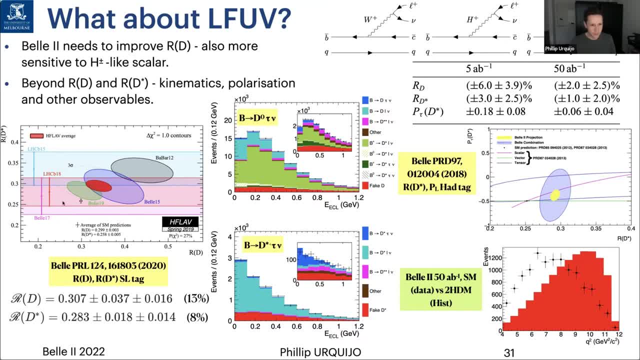 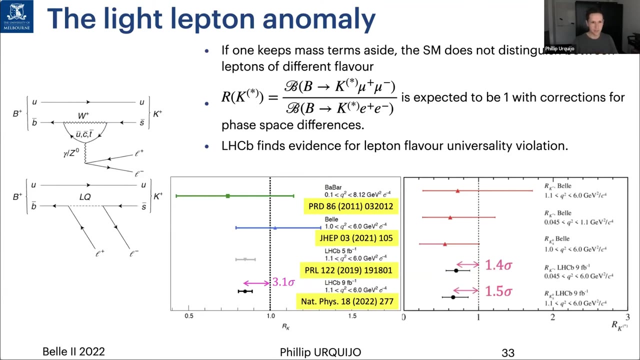 once you've got more data. In any case, we expect these curves here to really be greatly reduced in size. RD, for example, is highly statistics limited and the systematics on the D star channel are also data driven. Okay. So what about the other anomaly, the light lepton anomaly? 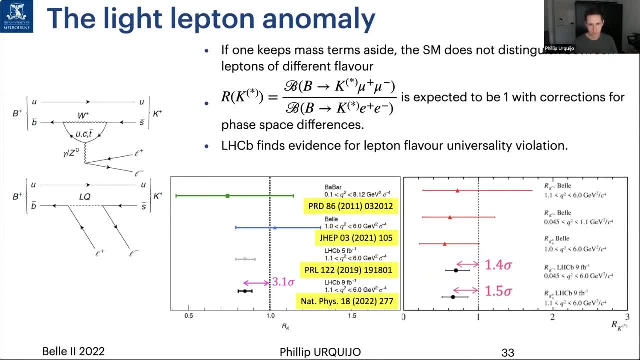 We've got RK star Now. in the case of the tau channel, it's clear to see that it's very challenging. You don't reconstruct the tau, you reconstruct the tau's decay products. Here you reconstruct the electron and you reconstruct the muon. 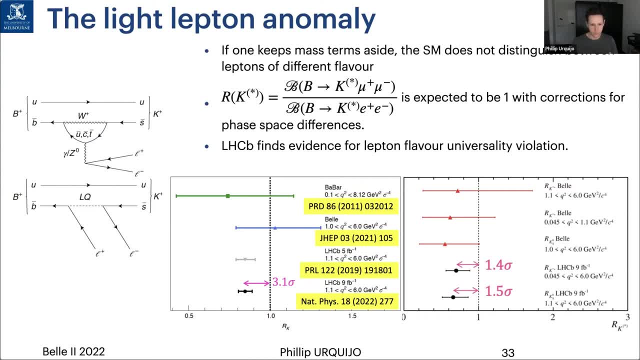 So you would expect it experimentally to have less issues. In any case, with corrections for phase space differences, the ratio should be very close to one, And you can see here a summary of the results right up to the most recent Nature publication from LHCB. 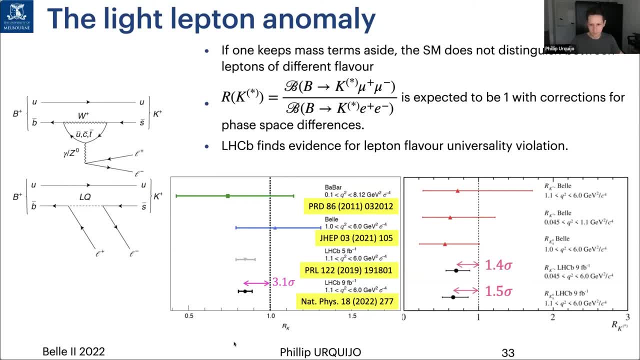 which is about three sigma away from one. The results on RK star, RK short through other channels are also away from one, although every result from Bell has been roughly consistent. So of course this could be some kind of leptochore, it would be, I don't know. 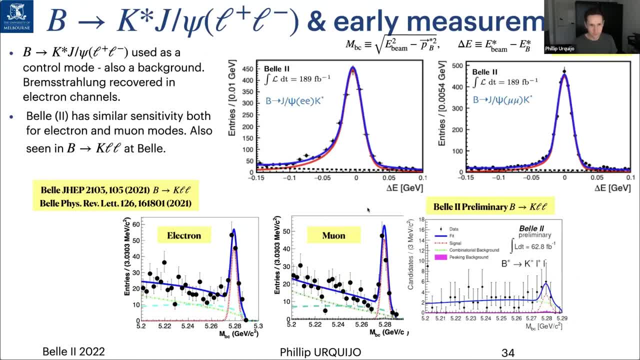 It would be some kind of new phenomena. So the early measurements: this is a highly statistics limited analysis. So the first thing you would do at a B-factory is look for a control mode, this case K star LL. So this is a preliminary result that just came out. 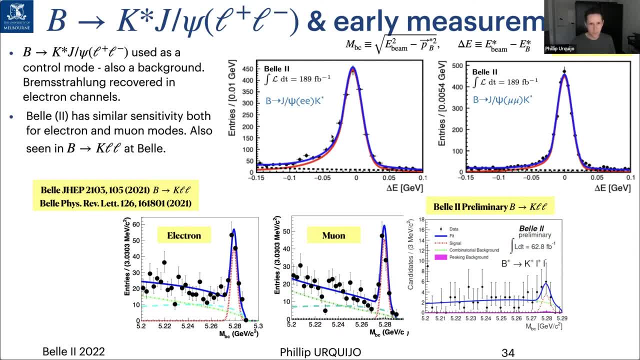 for which branching fractions are extracted Here: J psi going to EE and J psi going to be mu reconstructed. You can see delta E. they're very clean And the resolution of these peaks is really quite similar with respect to what you'd see at LHCB. 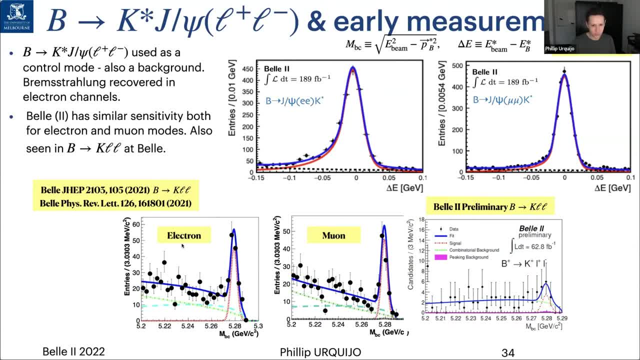 Same deal for the electron and muon modes. In that case we can use the beam energy constrained mass and the resolution is really pretty much the same. We're starting to find a KLL in the Bell 2 dataset. This was with a 60 inverse femtobarn analysis from last year. 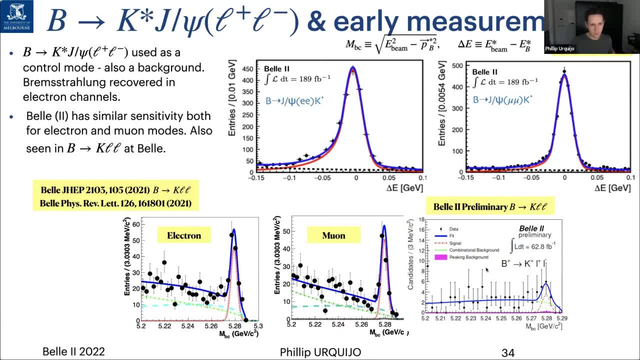 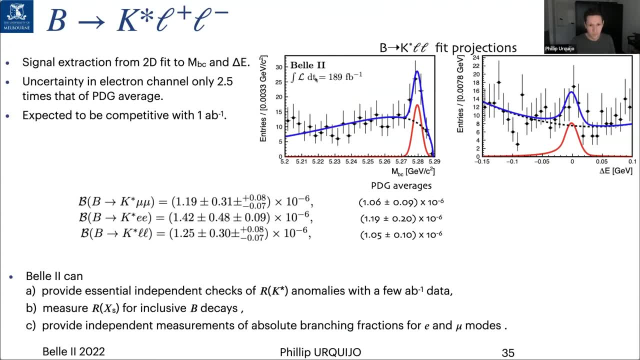 And it will take a few more years before we can make an impact on this one. And I'll go through those numbers. Looking at the most recent K star LL, this is with 189 inverse femtobarns- We were able to extract branching fractions. 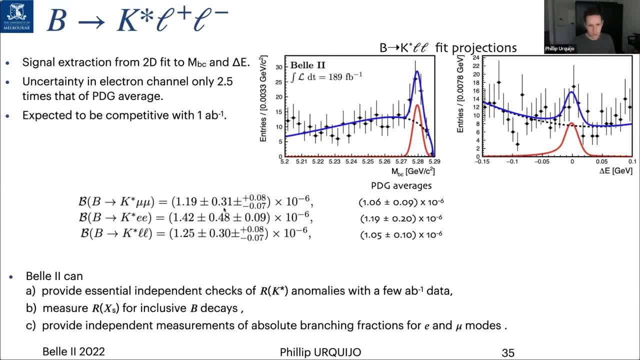 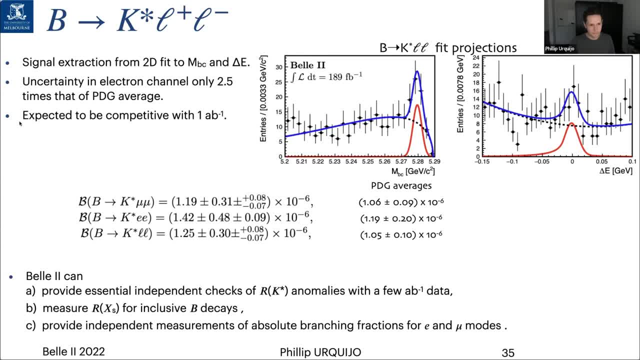 And the precision on these extractions is only around two and a half times That of the PDG with the small dataset. So for the branching fractions we're expecting to be competitive once we hit an inverse atobarn, that's five times the data. 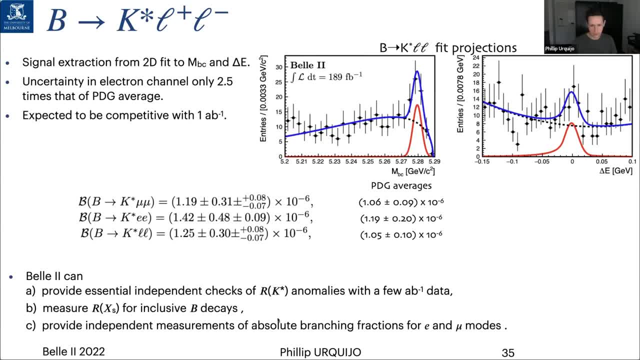 The main goal here is to give independent checks of RK, star anomalies and RK as soon as we can Measure the inclusive ones that you can't do at LHCB, And get some absolute branching fraction measurements as well to really start constraining potential subtractions. 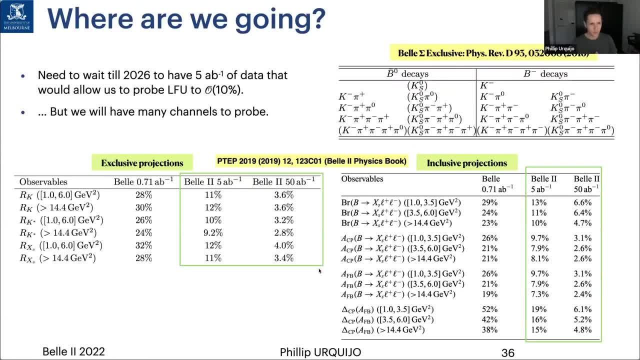 to really start constraining potential subtractions, To really start constraining potential systematic errors. So what's gonna go, what's gonna happen in the future? Here I've got some benchmarks where we expect that with five inverse atobarns. 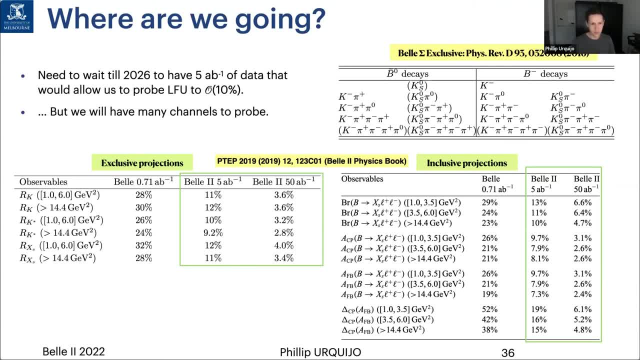 we hit 10% precision on all of these types of measurements, whether it's exclusive or some of it, some of exclusive or inclusive. This is probably gonna be around 2026,. hopefully We'll have a long shutdown in the interim. 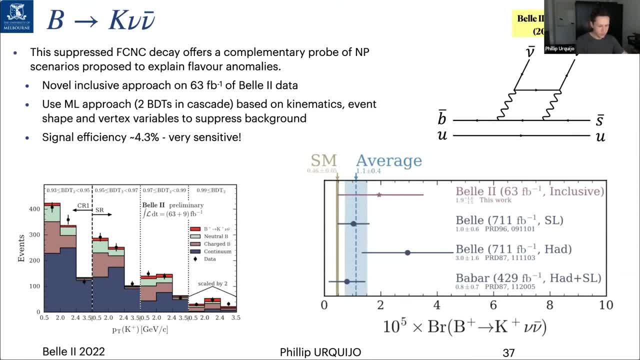 A great. so if you've got new physics in beta- K, star, LL- and you wanna find out really what it is and you wanna reduce your overall theoretical uncertainties, an excellent approach is to use the neutral modes. new bar: It's also a complimentary probe of new physics. 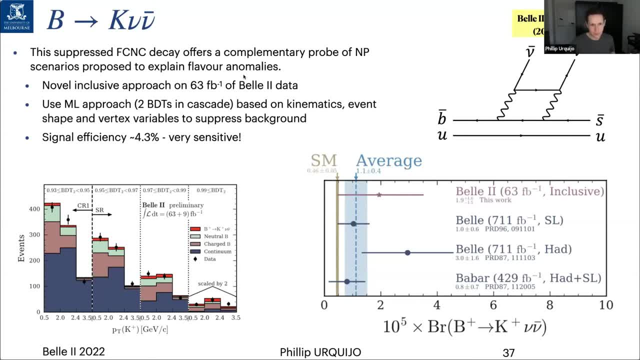 There's other things that can come in this one. So with around 63 inverse femtovans of bell two data. this channel was measured. It was published last year. It was by far the most statistically powerful per inverse femtovan of all of the methods. 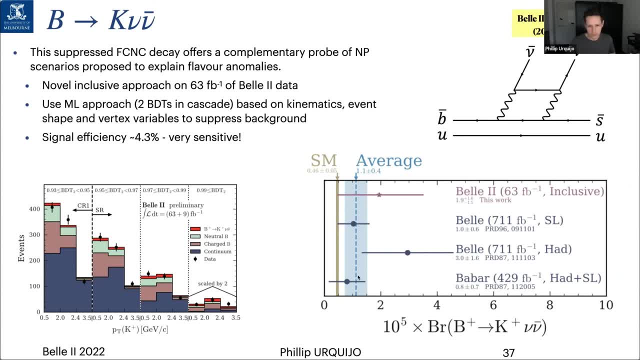 that have been applied And this is a comparison of the final results. This is the standard model, This is the average of the results so far and this measurement of bell two inclusive. So the way it works is it uses two machine learning approaches, so two BDTs in combination. 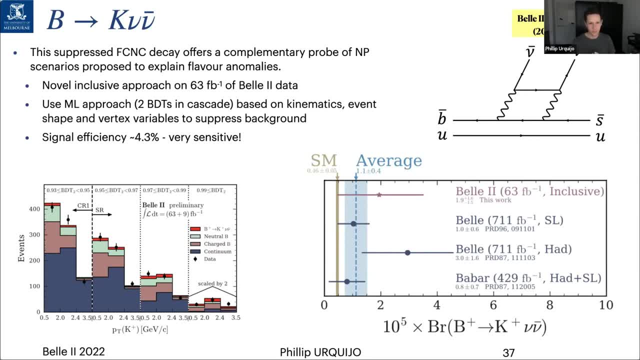 and it takes into account kinematics, event shape, vertex variables, all to suppress the background. and also some kinematics include the fact that K on this high momentum, et cetera, And this is where the signal comes in in red. 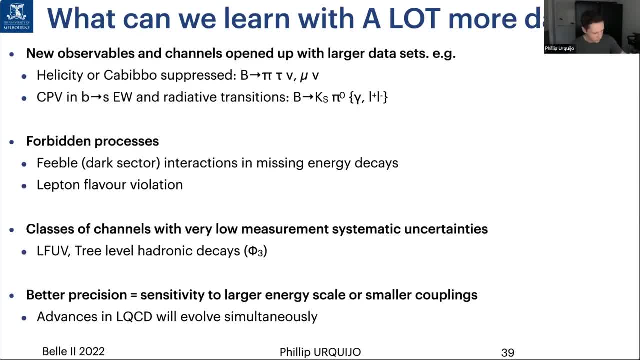 Okay, so what are we gonna do? Is there a reason for having more data or a lot more data? I've talked to you a little bit about what we're expecting, Let's say, in the next five years. that's around five inverse adobans. we're already starting. 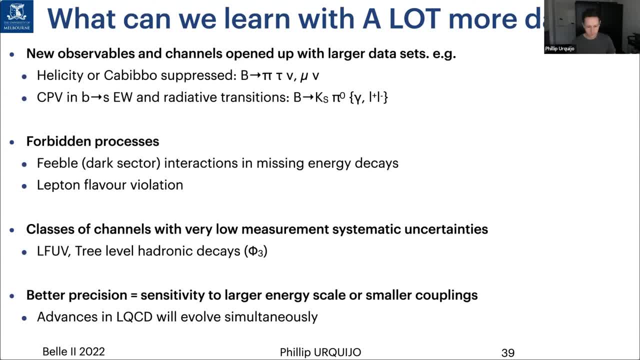 to think about. well, what's gonna happen beyond bell two? or at least can we make sure we hit the original target and then consider going on from there. but you need a physics motivation. So what can you do with a lot more data? 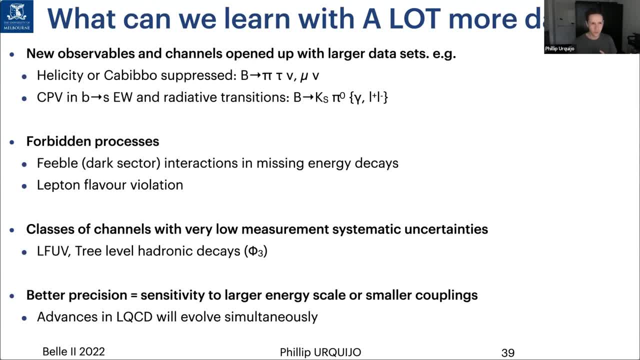 So I've broken it down into a few different areas. One is new observables and channels that you can actually do with more data. I talked about lepton flavor universality violation tests, where you can start looking at BTU transitions, not just B2C. 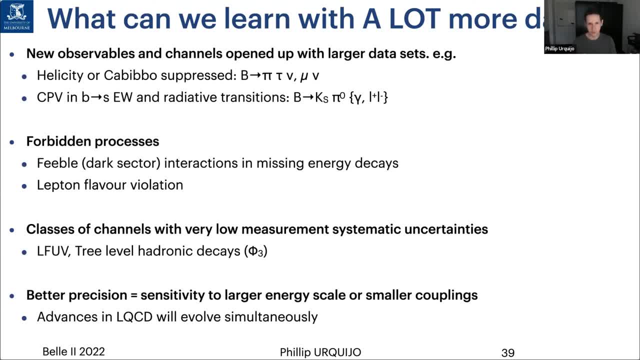 On Covibo suppressed. there are purely leptonic decays that to date have been either poorly measured or with no signal. yet B2M, you knew, is one in that latter category. Then channels that open up are CP violation measurements in B2S, Electra, weak and radiative. 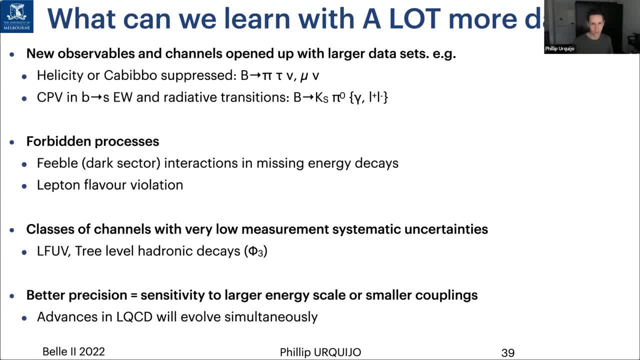 and to these channels that open up are CP violation measurements in B2S, Electra weak and radiative and radiative transitions. so these ones can be quite sensitive to right-handed currents. um, on next category, i would i'd say kind of forbidden processes or dark sector, so you can. 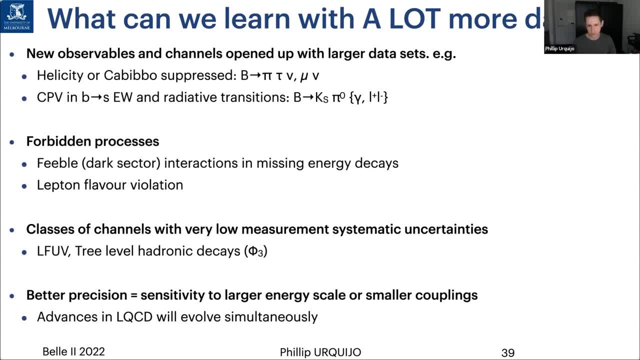 look for feeble interactions in missing energy decays. these are very often difficult to to really probe to, to to to new level without a lot more data and left on flavor violation, which offers very good value, um. third, one is on classes of channels that have very low systematic. 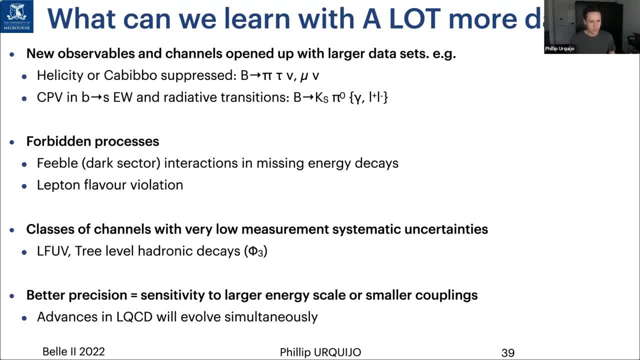 uncertainties or very low theoretical uncertainties. lfuv tests- so ratios of electrons and muons- are typically completely data driven, but there's also hadronic decay type measurements like phi3, which will continue to improve well beyond 50 inverse at advance, and i should also mention that um 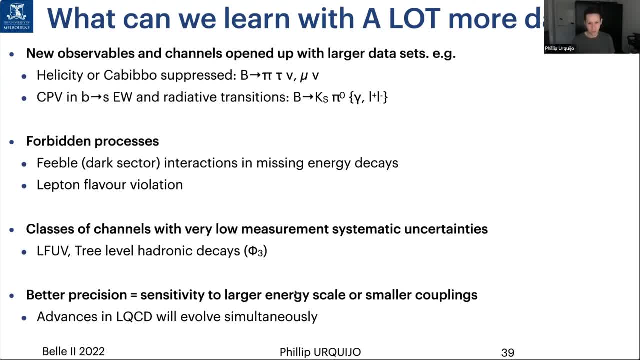 you know, once we achieve better precision, of course we can measure larger energy scales and smaller couplings, but you can't do it without improvements to theory um. at the same time, we're expecting that the lattice qct inputs on form factors, bag factors, decay constants will evolve according to their to. 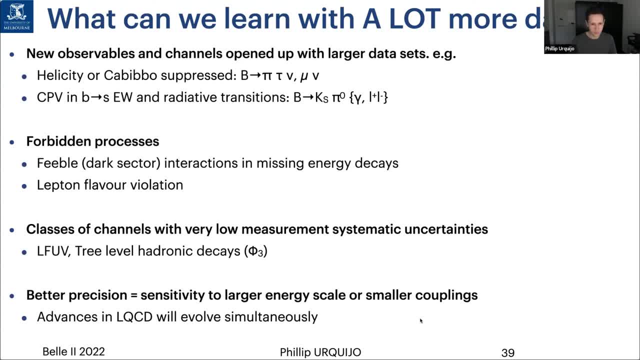 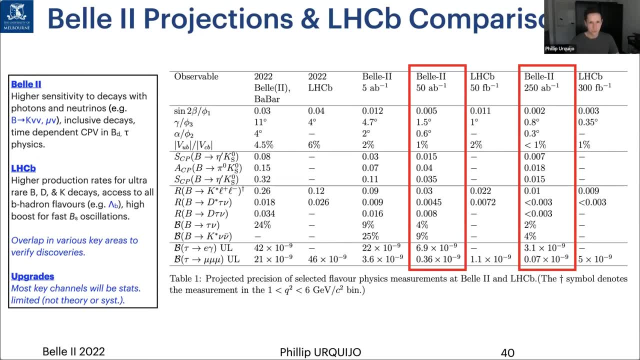 the stated schedules of the lattice groups, and that's really fundamental to saying that even on the hydronic side things will improve. so let's look at the belt 2 projections and the comparison between belt two and lhcb. so the first part of the today's talk was on cp violation. 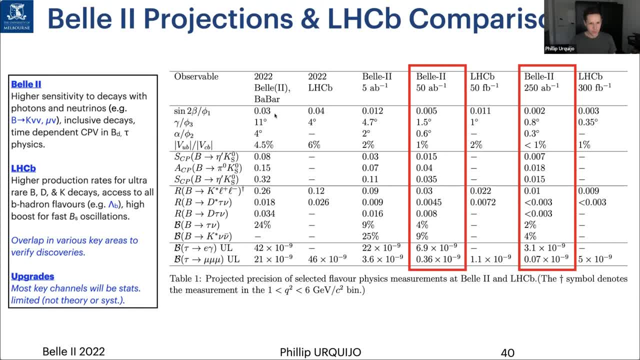 and roughly the the current state of state of a state level of precision from b factory. so i showed you, for example, that 5-3 measurement from belen baba with 50 inverse adobons. we're looking to push that down to around one and a half degrees and with five times more. 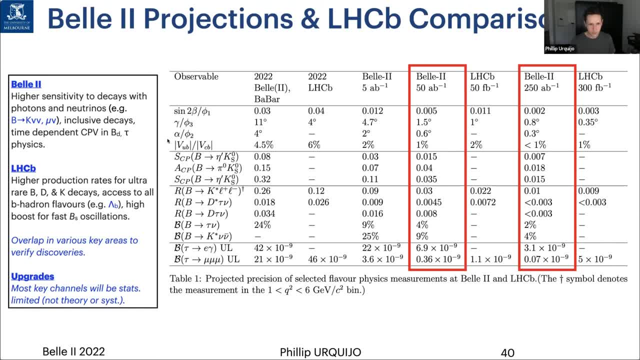 than that, well, well below one degree uh phi two was at about four degrees and this is statistics limited and will continue uh to just improve according to our expectations. ccam matrix element measurements, uh ratios, as i said, are good ways of cancelling theory errors and experiment errors. this will go. 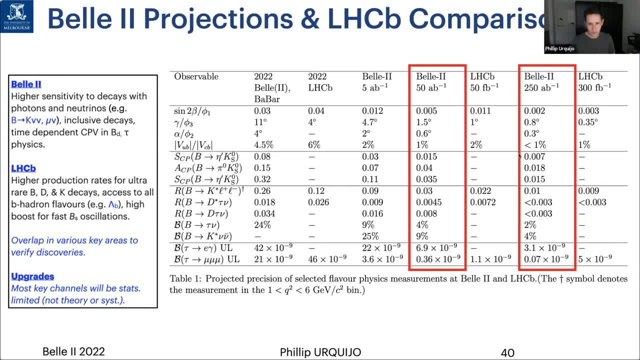 well below one percent and continue to do so. so ccam precision measurements are a really good argument for for a new experiment, searches for new physics, a cp violation in new physics. sorry, new physics and cp violation. um, all of these are very highly statistics limited. if you look at look. 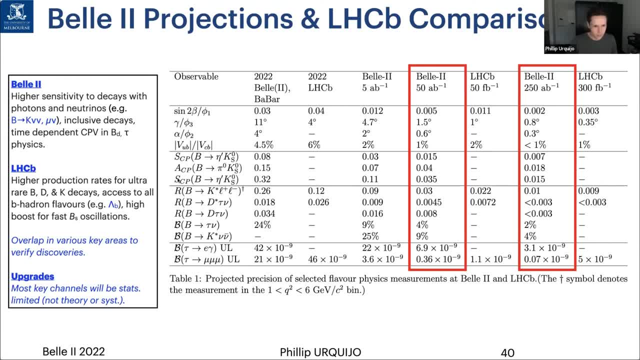 look closely and that that's a typo. okay, so in this one we've got uh searches for our kind of anomaly channels, and also beyond that with purely leptonic, i think, a highlight for the long term. uh, are these two so beta town, new um, where i currently have a precision of 24 or so? uh, it's clear that this. 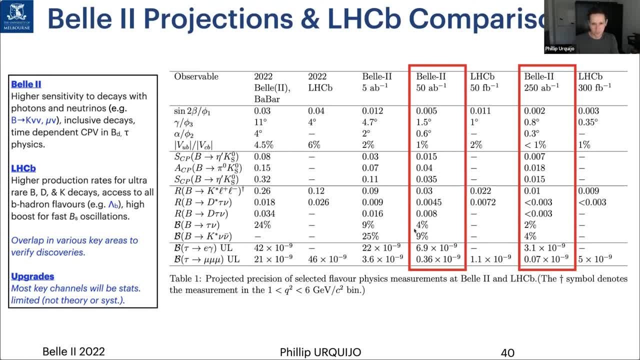 is not going to make a big impact at 24 um, but once we're able to push it down to somewhere between two and four percent with the upgrades, uh this will be significant. uh, in the case of beta k star new bar, that becomes a very high precision measurement. uh, once you push beyond, 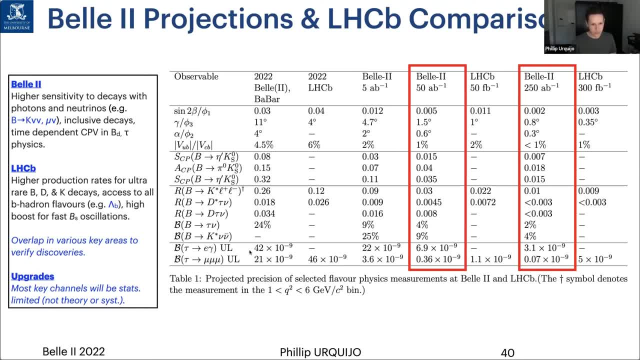 50. inverse adovance: uh. and then finally on this table: uh, lfv. so lfv left. on flavor violation: uh, generally in many channels are zero background tests, so you can push down to levels of 10 to the minus 11 in this case. just to give you an idea of what these channels look like. 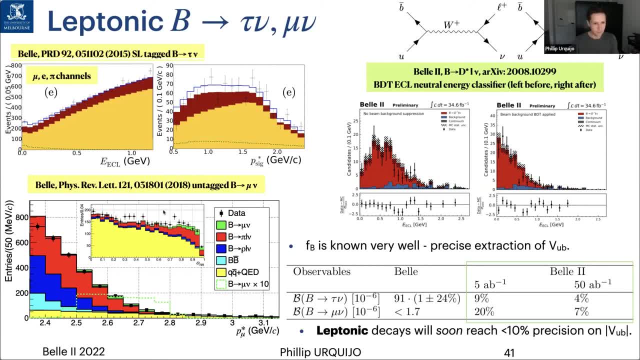 this is beta tau nu and beta mu nu in the full bell data set: mu nu, which is green, and the left on momentum, and you can quite clearly see this is a very challenging measurement. you need a lot of data to get to. in the case of beta town you, this is what the signal excess looks like. 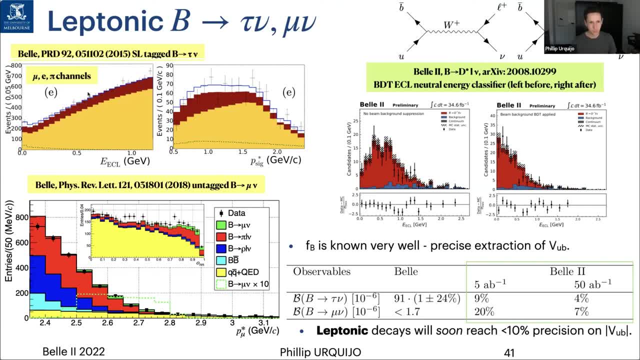 again, more data will give more, more handles on reducing this background. i'll not go through the details here too much, other than perhaps just this last one. leptonic decays, other than looking for new physics, are an excellent way of looking at the background of the signal, and the signal and the 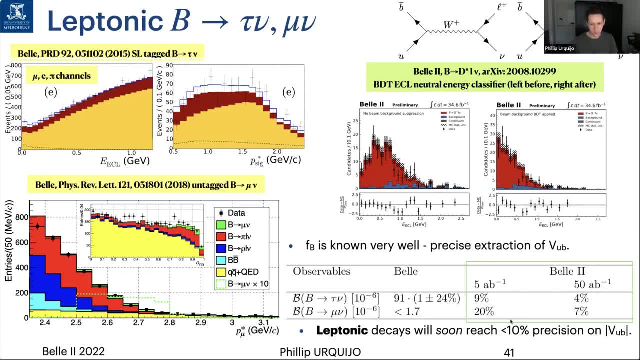 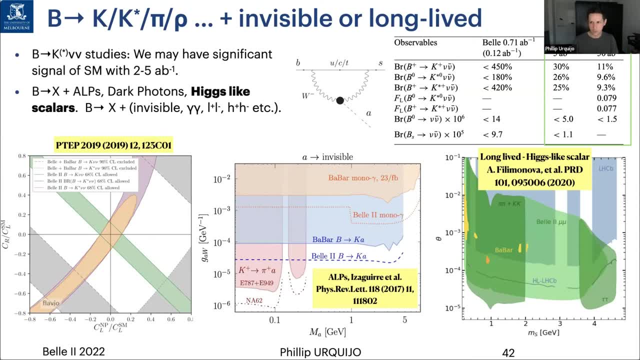 large field of the signal we're looking at and we'll be looking a little bit more closely at this. here we can actually see the linear velocity session of the signal and the inned value in the patc, known as k-ians for this problem, and we'll be looking at this next little. 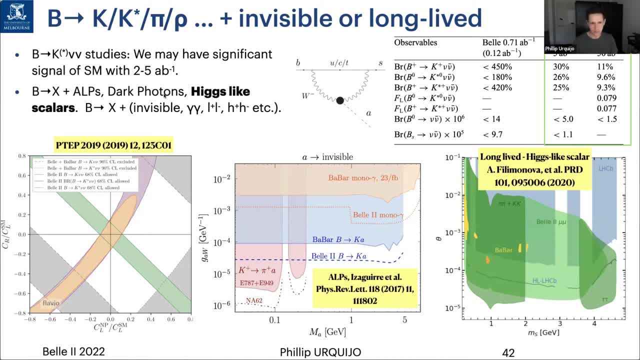 piece. there we'll be looking at the linear velocity of the signal that we're looking at now in relation to our essentially the linear velocity of the signal in the first generation. over the next couple of years we're going to be looking at a particular way of getting out c cyma matrix elements and that will actually work exceptionally well in the future, since decay constants have determined very well. another thing i'll just flash because i'm running out of time, and this is searches for dark sectors, a really good motivation for future analyses. so we've talked about k and k star new bar. but the same processes could be harboring axion-like particles or dark photons or heaps like scalars. that 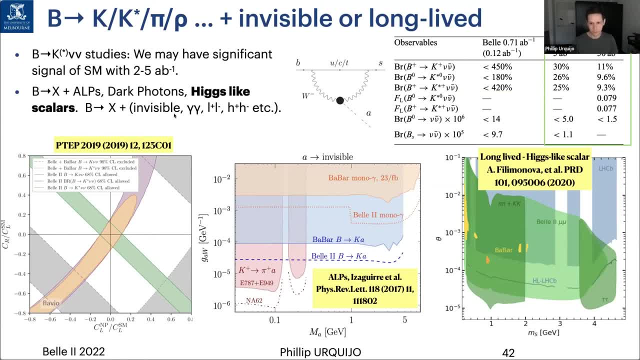 are invisible or long-lived, and there are many ways to probe for these that are being discussed in the literature. at the moment. it's actually one of the hot topics, i think um. so once we push down to precision levels, um, we really start constraining new phase space for for these kinds of models. 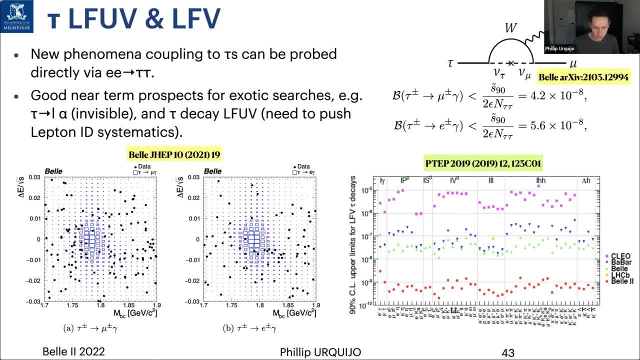 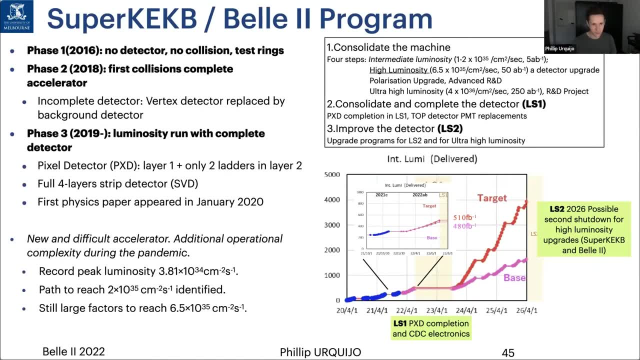 uh, lfuv and lfv, i'll i'll actually go past this one because of the time. i've got to go through this one as well. okay, so let me get to the. so the super tech b and bell 2 program. uh, so what's happened so far? uh, phase one was in 2016. there was no detector. phase two: 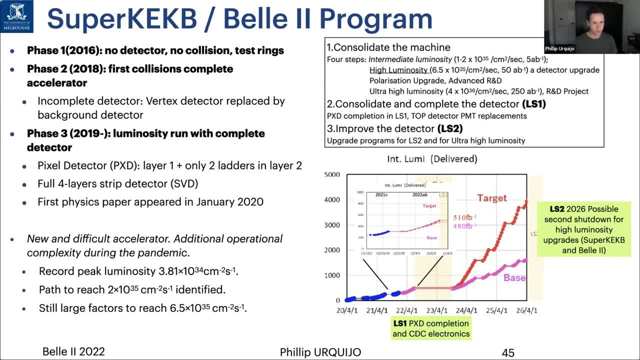 we had first collisions and pretty much a complete detector, except for the vxd that was partially incomplete. sorry, i misread this one: first collisions, complete accelerator and an incomplete detector. uh, this uh meant that the vertex detector still had the background detector in it. it was 2019 that we had the detector with the one layer pxd. 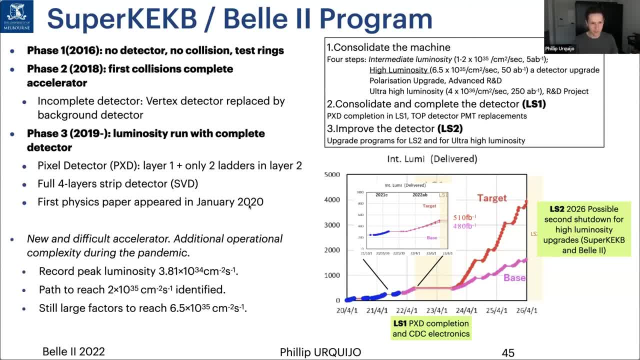 um. so we had physics papers come out pretty soon after that, in 2020, but it's been a new and difficult accelerator to work with um. you might have seen that some of our projections for expected integrated luminosity haven't quite hit the mark. on on on what we were. 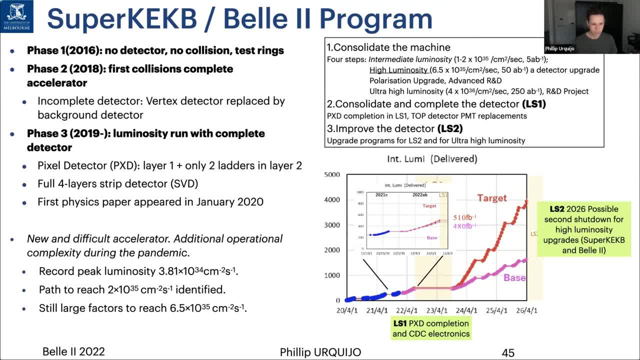 expecting to have by this time since we started. and again that's due to complexities, it's due to operating during pandemic etc. so the peak luminosity already is getting to the super kick b levels. the plan to go a factor, a few more than this is identified, but then to go. 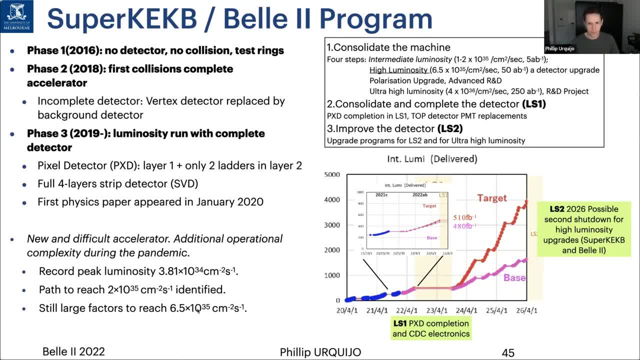 right to the nominal luminosity is still a challenge. so there's a program for this on the machine level to get to that intermediate luminosity and then move to high luminosity. uh, there are plans for uh consolidating and and completing the detector, So this is coming up. shutdown will involve installation. 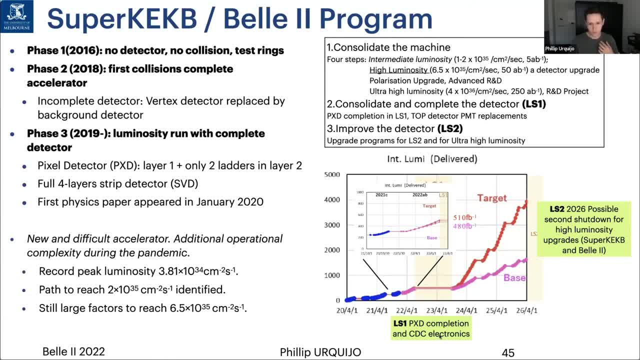 of the pixel detector, second layer, and upgrades to the top detector, PMT replacements. That was a typo. And part three would be to improve the detector And that would be in the phase over here, essentially the long shutdown too, And this is the kind of preparation. 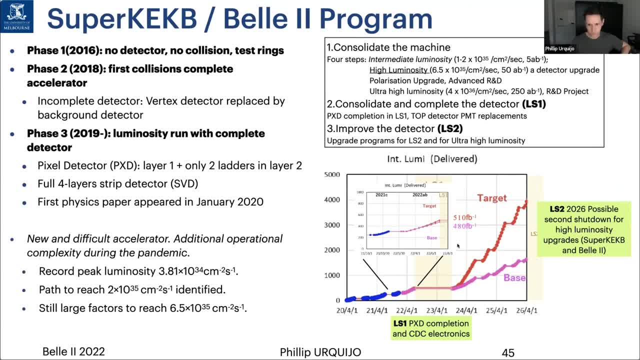 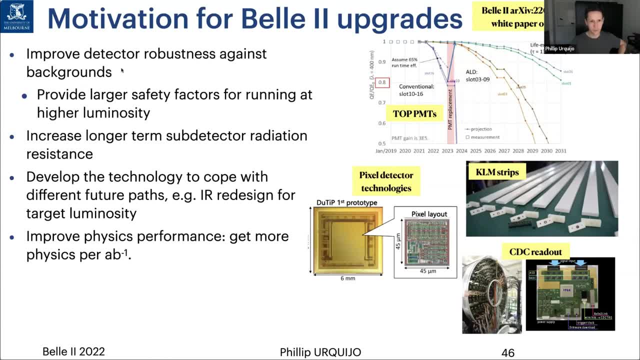 for that high luminosity scenario. So what are the motivations? These are written up in a SNOMAS white paper on this. Firstly, to improve the detector robustness against backgrounds and to have better safety factors for running at higher luminosity for some detectors. 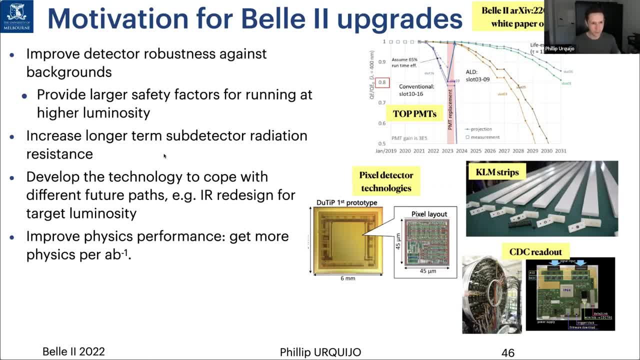 Many of them can be affected by higher radiation levels. So radiation resistance is important, And then to have the technology work very well if the interaction region needs to be redesigned for even higher luminosities, And my favorite one, which, of course, is to improve it. 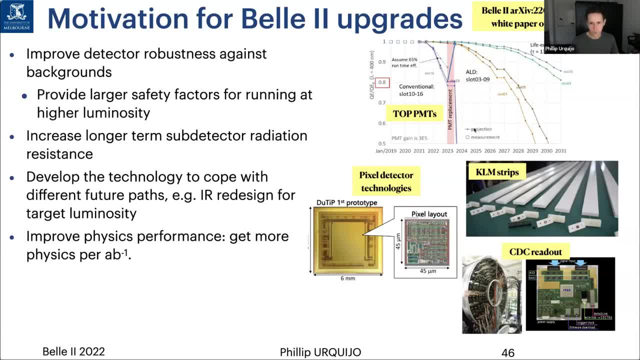 just to get more physics to invest out of bonds. So the top detector replacement I just mentioned is a replacement of the photo multipliers. This is required because their efficiency drops off after irradiation and they're being replaced with ones that will be more radiation hard. 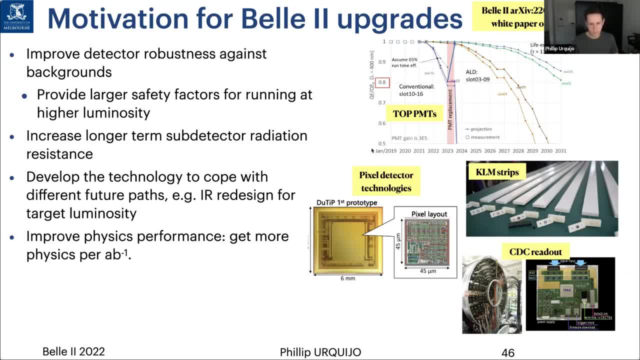 Other detectors are coming in, such as, or are being discussed, such as: new pixel detectors for improved performance and robustness in the inner region, upgrades to the KLM strips on the outer region of the detector and upgrades to the CDC readout. This picture gives a bit of a rundown of all the areas. 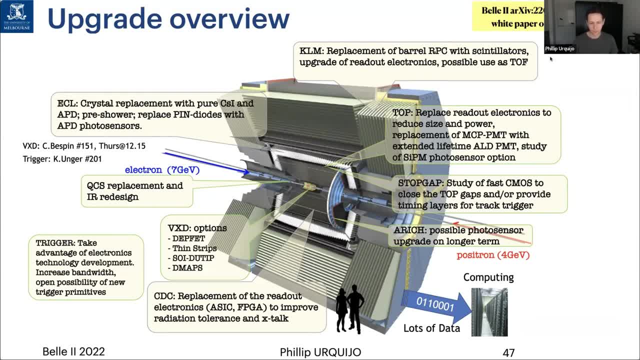 that are being considered as part of this write-up. Not all of them will go through, but the discussion is currently open to understand. Thank you. So the bunch of options for pixel detectors: there's going to be upgrades associated to the trigger to allow better bandwidth. I mentioned the CDC upgrade for improved readout, so this: 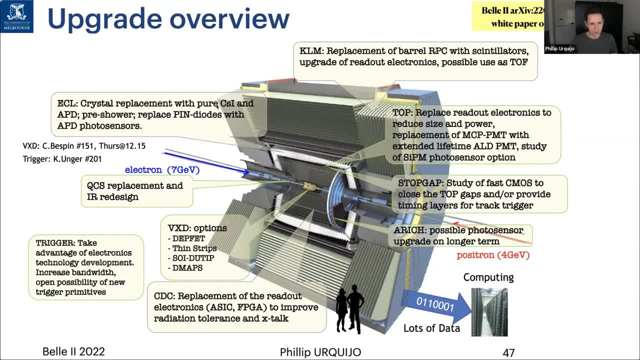 improves radiation tolerance. The calorimeter: there is consideration for pure cesium iodide in some parts and to replace the photo sensors that are there with these avalanche photodiodes. On the KLM side some of the layers still have RPCs and it would be to replace them with. 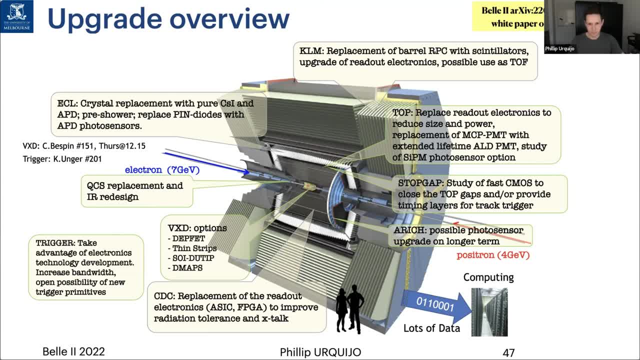 scintillators On the top side I mentioned. and then there are some areas of novel R&D, such as stuffing all of the gaps in the particle ID acceptance with high performance detectors so that you improve your vetoes, and so on. And yeah, that's for those. I'm not going to go. 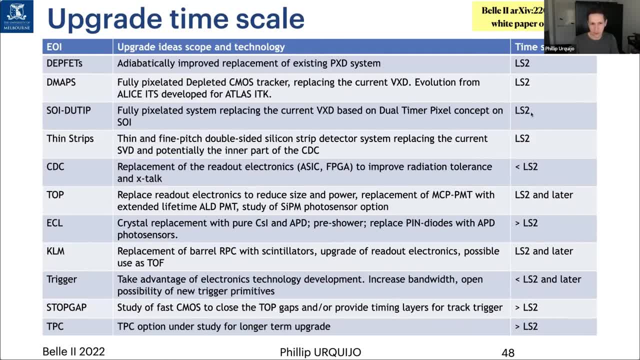 through this one too much. The idea here is just to show that a lot of the upgrades that I've just talked about are either in that second long shutdown- so around 2026, or at least nominally in this plan, or in some cases. 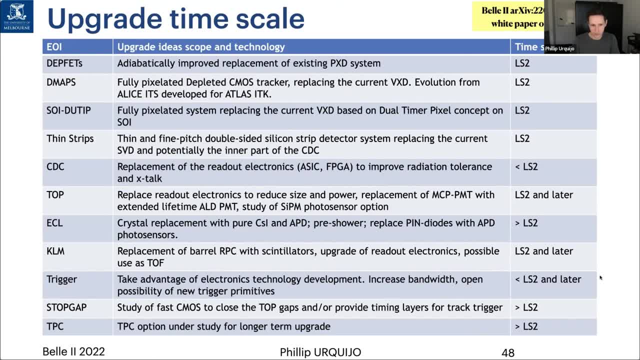 they'll be just before it in the case of the CDC, and that there are some that are longer term: the calorimeter and some of these at the bottom here. So that goes from transitioning from purely BELL2 program to you know the BELL2 program. So that goes from transitioning from purely BELL2. 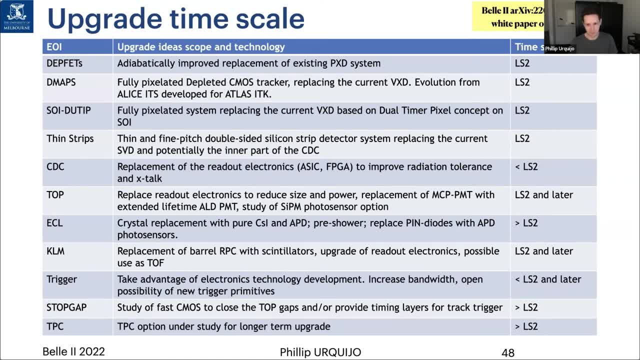 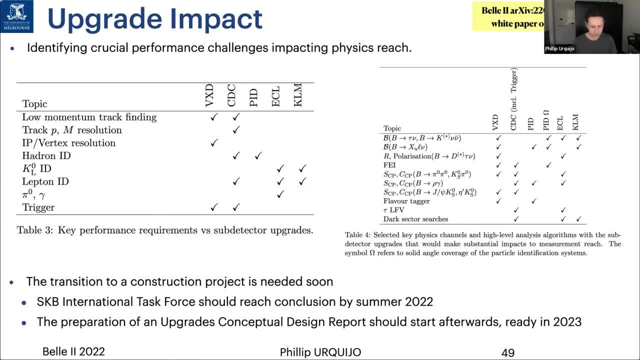 program to a BELL beyond BELL2 program And just to state that a lot of the perform, you know, these upgrades have to take into account what their impact and the challenges will be for different physics areas. So each one of these detector upgrades will have an impact in different. 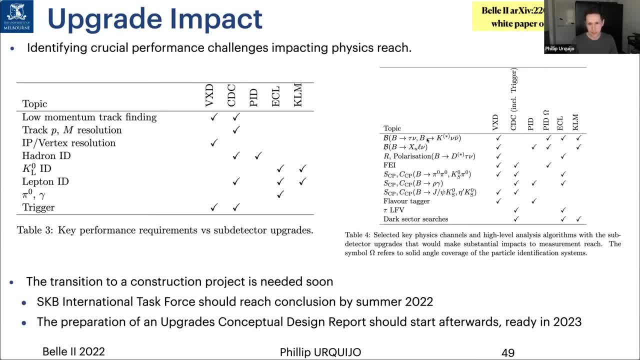 areas of performance and hence they'll have different impact on different physics channels. So there's now we're in a period of transitioning this to a construction project, Once the SuperCACB International Task Force reaches its conclusion about its plans. then this, the upgrade conceptual. 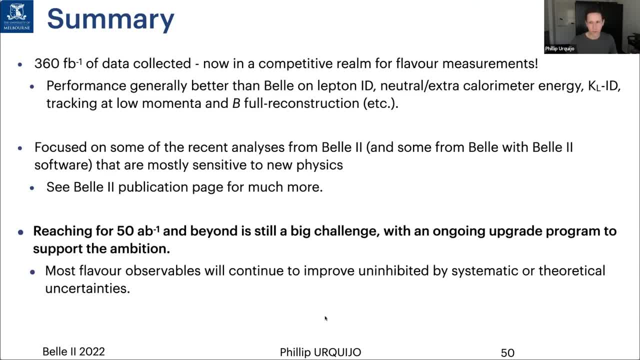 design report will be written for the program. Okay, that's all for me. The data set's actually quite large already: 360 inverse vanterbahns. Performance is doing generally as good as, or better than, BELL2.. BELL1 and BELL2.. 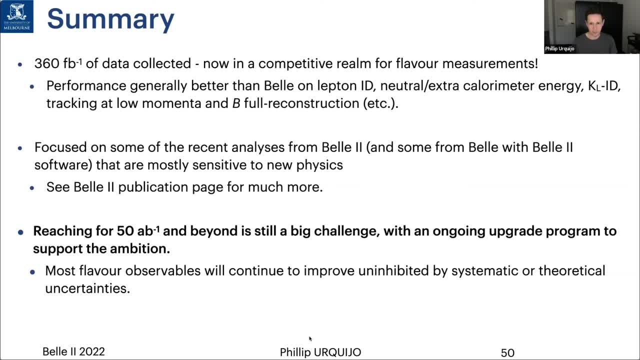 BELL1.. I showed you some highlights, plus some from BELL, and exactly how we can get to 50 inverse vanterbahns, which is going to have to include some types of upgrades as we go along. Okay, that's all. 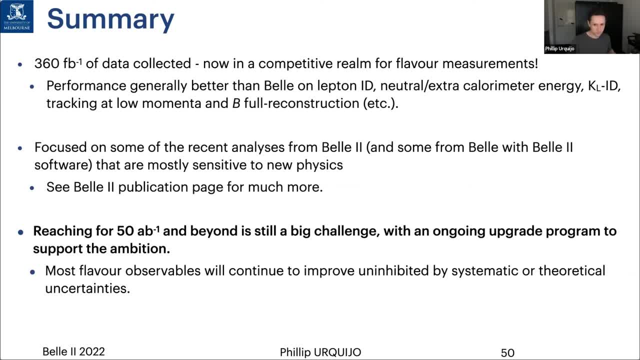 Thank you, Phil. That was an excellent talk and I learned a great deal from it. So your talk is now open for questions or comments. Can I ask one question, Tom? Yes, please, I can barely hear. Yes, somebody wants to ask a question. Please proceed. 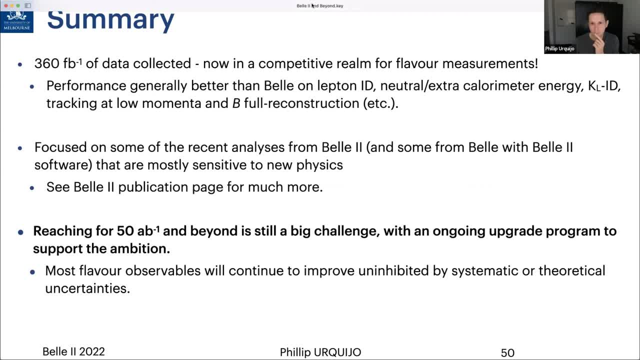 Yeah, Thanks, Philip, for a very interesting talk. Your volume is so low we cannot hear it. Okay, Let me adjust my volume. In the meantime, somebody else can ask a question. Let me just adjust, Okay. Next question and then we'll go back to whoever is speaking first. 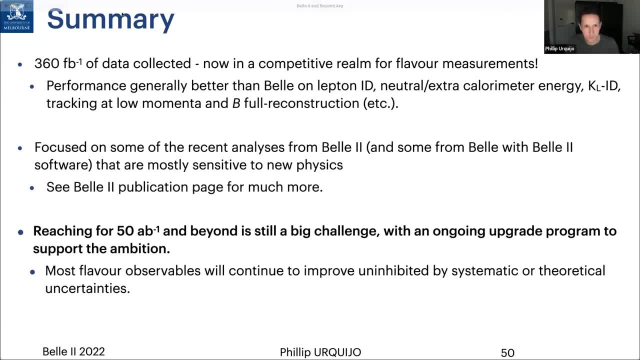 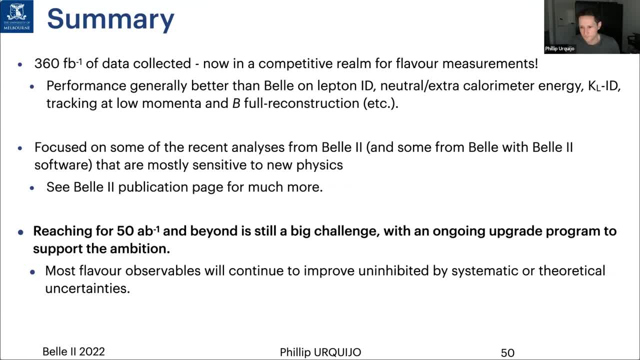 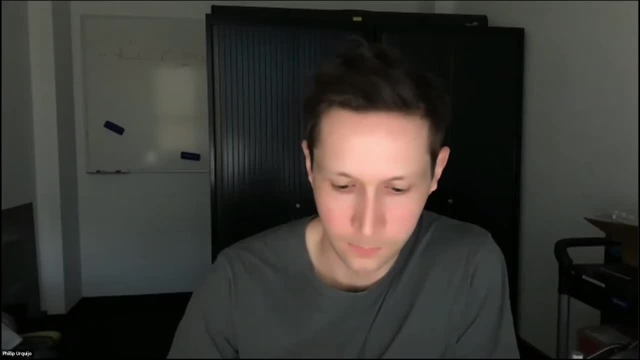 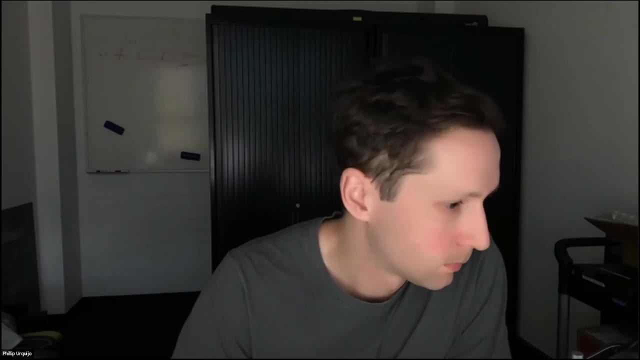 is okay. please proceed now. Hello, Philip, is it better now? Can you hear me? Yes, Okay, Yeah, So I have a question regarding inclusive decay. So if one considers B2U-LNU inclusive, is it possible to also look for an additional? 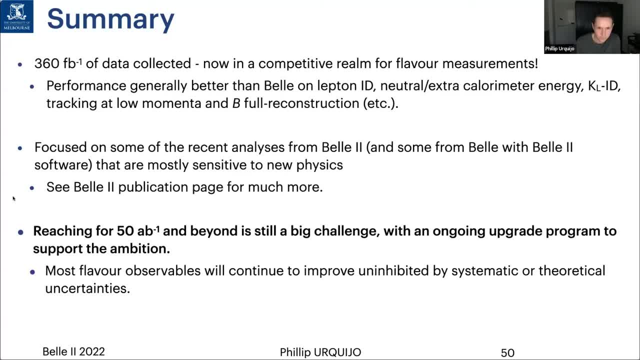 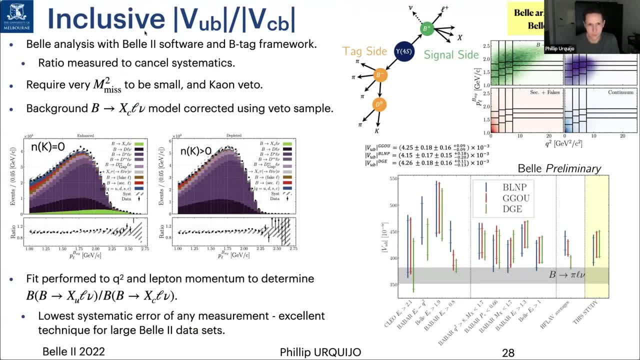 hard photon with this kind of a decay. Sorry, I had my mic muted. I think you were talking about this channel. Is that correct? Yes, Yes. So my question is: can one look at B2XU-LNU and a hard photon? 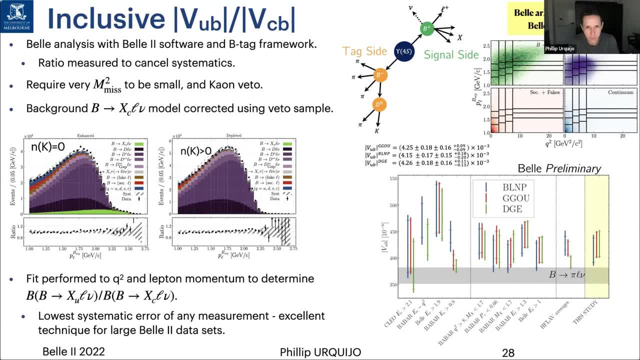 So a high energy photon coming out, and what would be the motivation for that one? I guess you could, but it's a little difficult, right? Oh, okay, No, So motivation was we were just trying to look at how to extract the non-perturbative parameters. 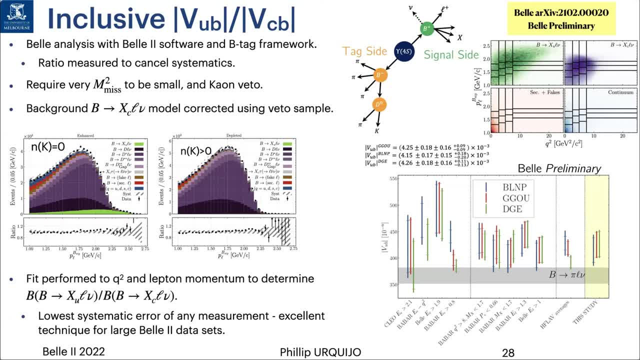 and it looks like we have not completed the calculation, but it looks like that there may be a useful thing, Because from the very preliminary results that we get from calculation, it looks like there may be a useful thing. Okay, So if we are computing one part of the rate, looks like that some of the non-perturbative 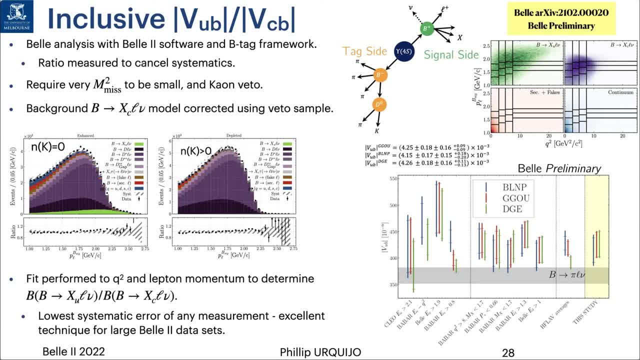 parameters can come out more cleanly, at least theoretically. We have not completed the calculation, So that's a caveat. Yeah, So this probably comes to the method. When you do this analysis, you reconstruct this X system. you reconstruct the invariant mass of it by looking for tracks and for photons. 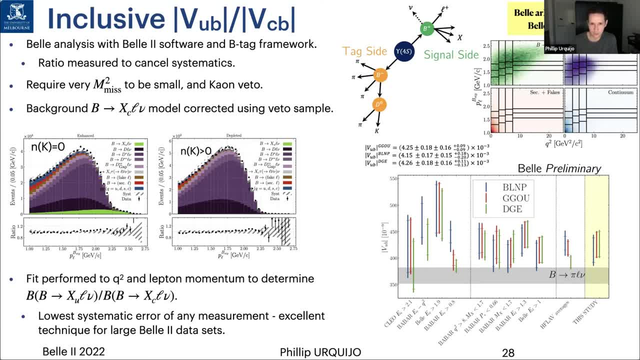 Or pi zeros in that part of the event. Normally we look for everything and if it has a significant amount of momentum above some detection thresholds then we'll include it in the four vector of that X system. But typically we don't normally break. you know, we don't normally search for a high. 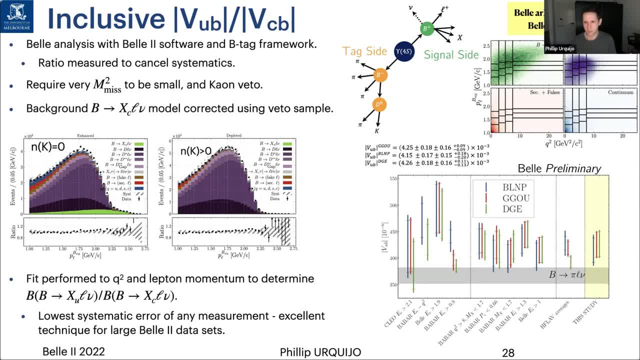 energy photon component in there, I guess largely maybe because it could come from a pi zero, So that it hasn't. but if it's an interesting proposal, I guess we can see what could be done experimentally. Okay, Thanks, Okay. 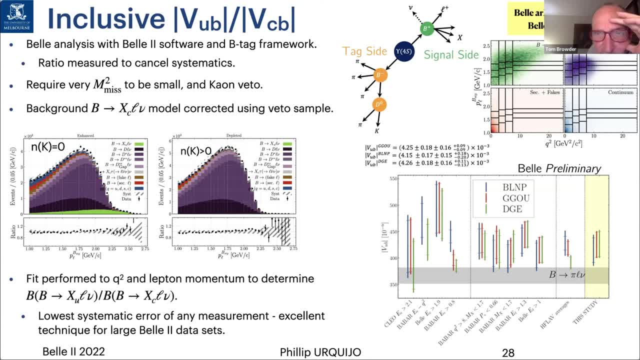 Next question or comment If I don't hear one right away. I was, I think. earlier in your talk you zipped through the dark sector work, which I think is of great interest, So maybe you could- Maybe you want- to show the two slides you skipped. 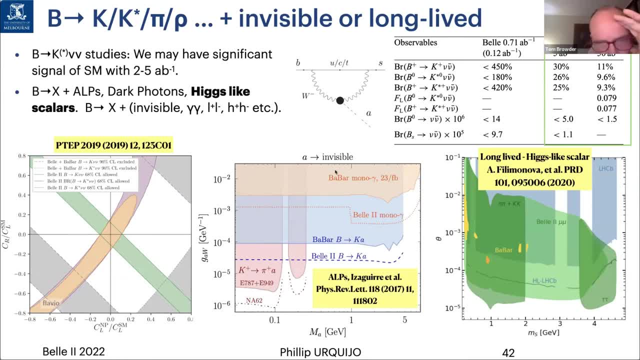 I think it could be this one. Okay, There are the two. there are two channels that I've got here. One of them is looking for B2 kaon plus an ALP, where the ALP decays invisibly. This was a theoretical analysis and it was a reinterpretation of the Babar search of. 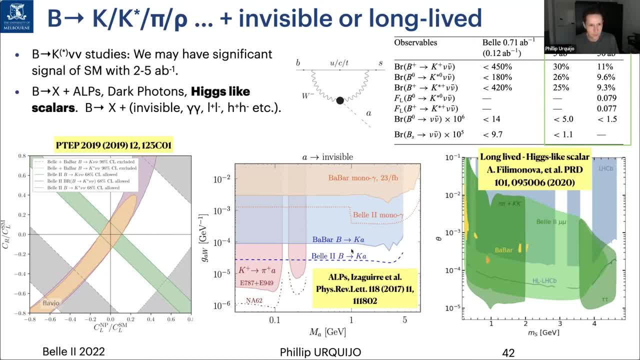 the K in a new bar. The principle here is that the, the ALP, will have some specific mass, And if you scan for the recoil mass of that out, then you're able to determine its presence, since the background will be completely flat. 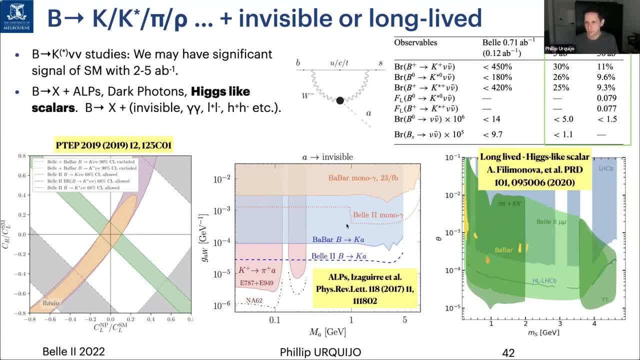 So that can be done in the K on channel, the PI on you can look for proton ones, for looking for Barry on it Dark matter. There's a whole bunch of categories that you can do here. We've actually done some Sensitivity studies in with, with with Bell and bell to MC. 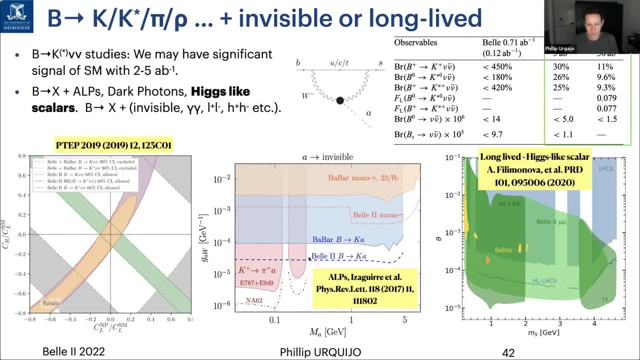 And we've actually found that where it's labeled bell two for the full data set is actually not quite so correct. That's what we expect with what we've got already, So bell two should be able to go well, well beyond that. On the one on the right, it's a channel involving Higgs like scalar. 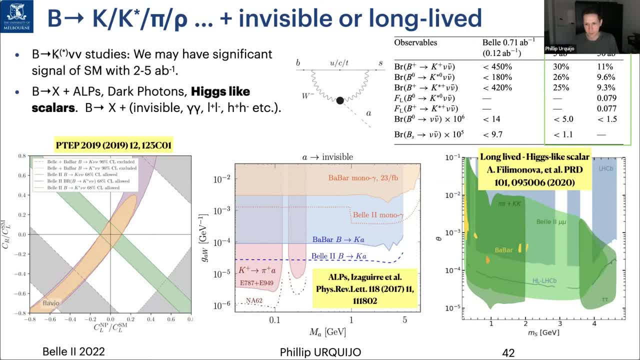 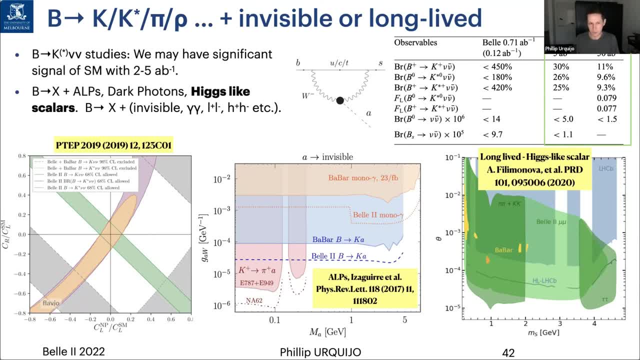 can have a displaced vertex, So it will decay after some period of time. It's showing three, three regions: one where it's reconstructed in the dime, you on Dietel Or a diet John final state. you do the same, you do something similar, but in this case 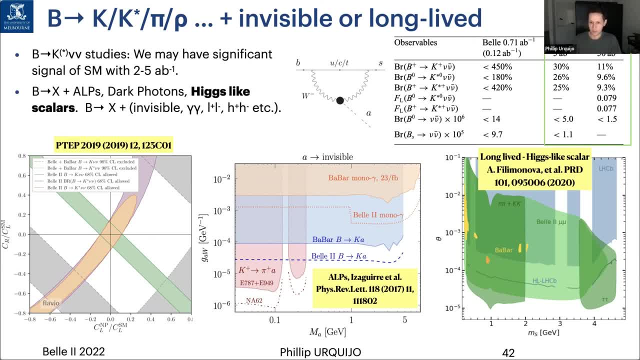 you're looking for a resonance peak with a large displacement, and it's been evaluated that that Yeah, Because of the relatively low momentum in Bell 2, you have a slightly better sensitivity to this coupling space versus mass, because it doesn't boost outside of the acceptance of the detector. 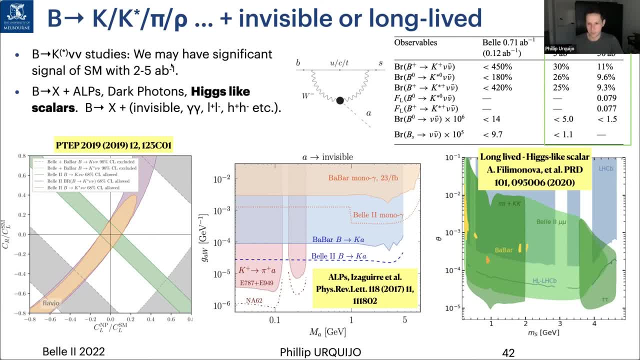 So this is quite promising as a category of measurement that Bell 2 will come out with in the future. Okay, so let's see the dark sector. stuff you talk about here is from BDKs, not directly from E plus and minus. 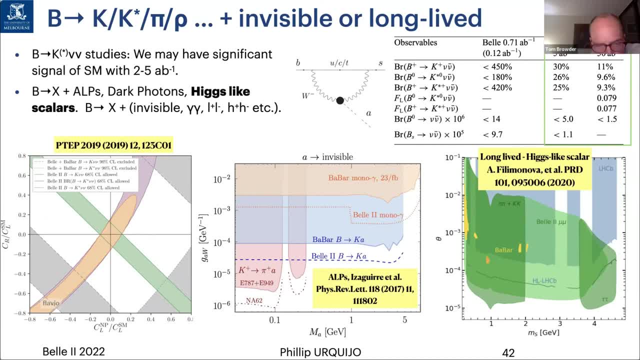 That's right. yeah, We have a great deal of activity on that front too. Yeah, I guess due to the name of the conference, I kept it to these topics. but yeah, I don't think I've got any. I don't think I I don't recall putting slides on that in this presentation. 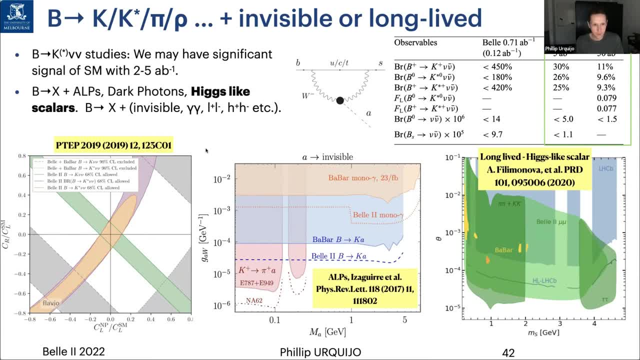 But yeah, you can do complementary things And in In those. in this case, if you look, the coupling here is between the ALP and the W. If you look in the scattering processes you might be looking at ALPs coupling to something else. So they provide complementary inputs. 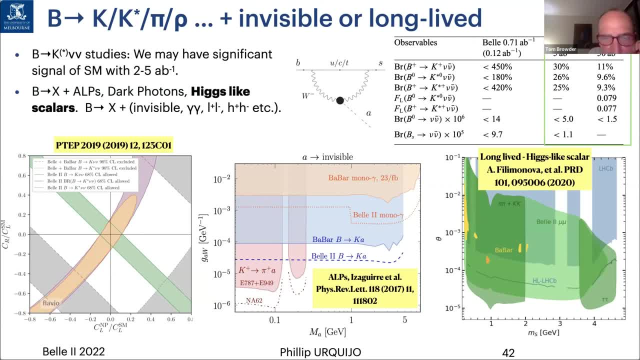 Okay, so let's continue. Maybe some other questions have developed since since you showed the slide. Can I ask a question here? Sure, This was. thanks very much for asking him to show these two slides, because I find them also very interesting. Now, the question I had was this: is you, have you said that the Bell 2 limit should in fact go down in real life? 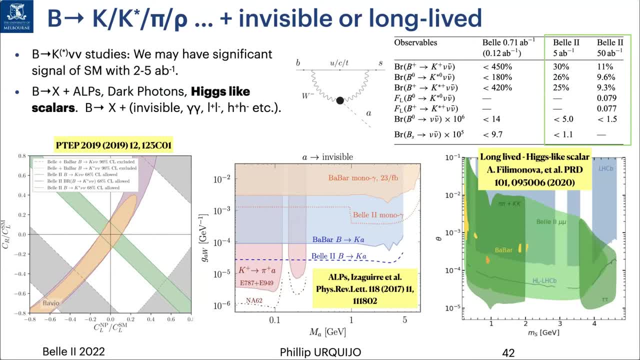 beyond what is shown in the central figure. So the for sort of phenomenologists, what would be your guide to tell how we can estimate that? I mean, is there some instructions to us for that? I'm glad that there were questions on this topic because my PhD student working on this exact topic to provide some kind of even Monte Carlo based sensitivities for these channels. So I'd be very happy to follow up if you'd like to afterwards. 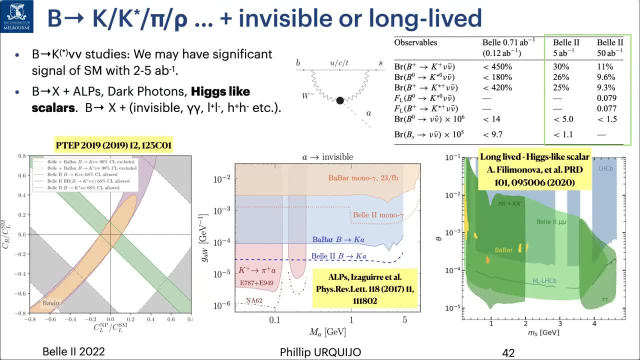 Okay, no, because I just felt that clearly you said the improvement is in the Bell 2, and that is going to be really because of some issues with, I mean, some betterment in the analysis, And for a phenomenologist to implement that we would need guidance from you guys exactly what we should put. It's not just a question of increased luminosity or something like that. 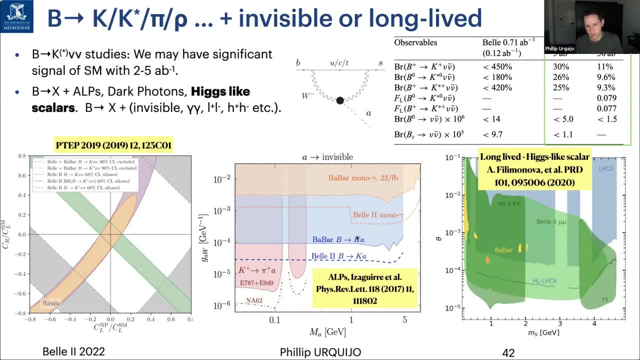 Yeah, So the way that the the previous measurement that was done by Babar was for beta k NU bar And then they binned their search in missing mass squared bin. So these are actually very wide, much, much wider than the recoil that you get from the ALP in this case. 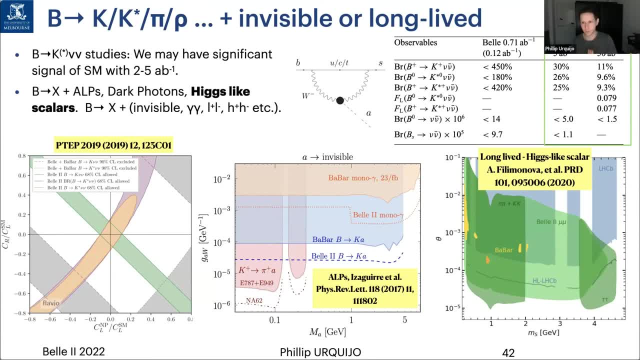 Okay, So a dedicated search can look in a much, much, much narrower window, and that's why the sensitivity is much better. Okay, so at least this is the physics reason. that would be there. Okay, Thank you very much for this. This is because I find it very interesting. if you are. 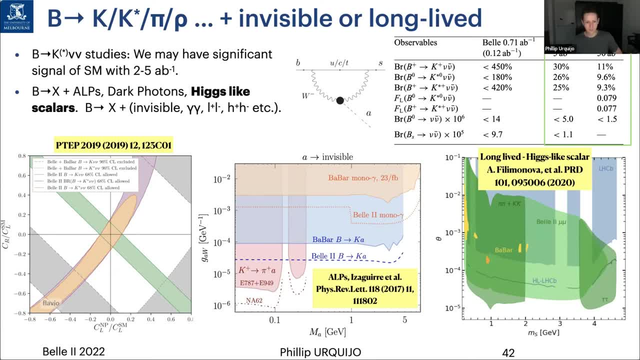 able to go down even further with Bell 2, so we're never, we're not going to get to the K on level, but we'll, yeah, it'll be better. It would be nice to see exactly where you go with this And then that would. I think a lot of theorists would be interested in this. 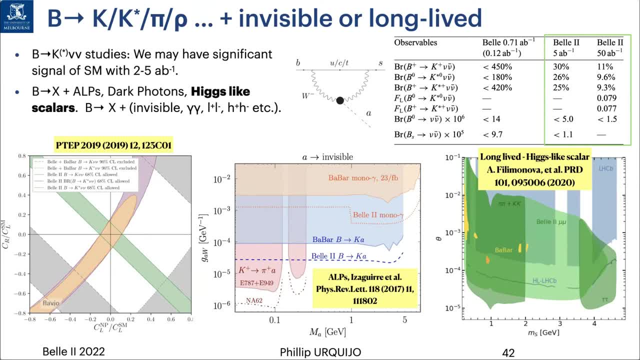 Thanks, Let's see if it's. if it's okay with Jim, I would like to allow for another question or two. Yeah, that's fine. The next talk is at another 10 minutes, So Okay, so let's continue Then. other questions or comments? 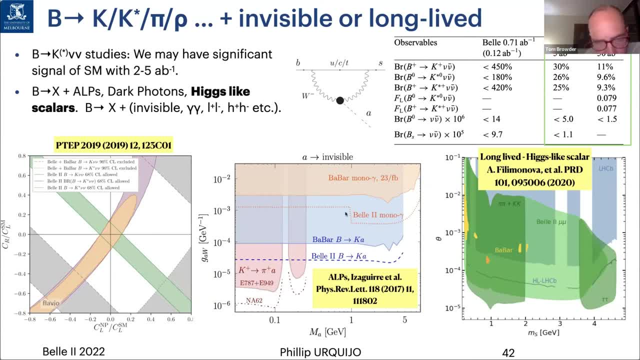 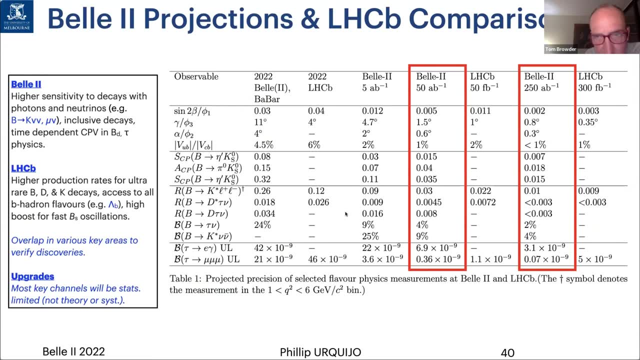 You had a plot- I think was around page 40- on the relative sensitivities and complementarity between LHCb and Bell 2 in the long term Future. So can you try to distill what are the strengths of the two programs and the complementarity? 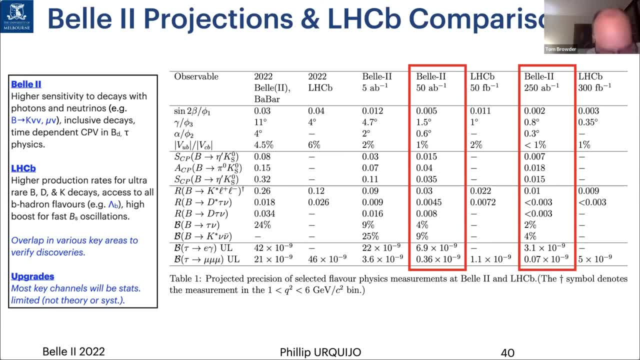 For Bell 2 and LHCb. Yes, yes, Right, It's, it's. it's kind of funny, this one. We have our prejudices on what we think we're better at, And so I've got listed over here. 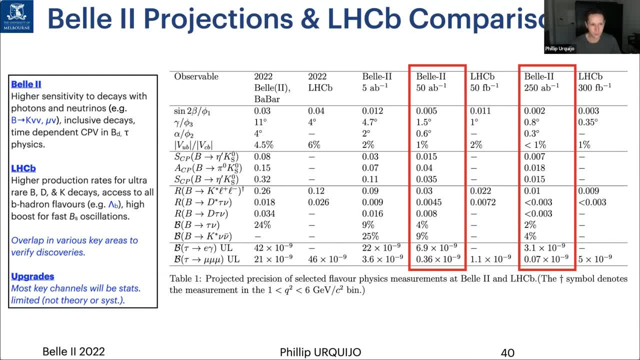 We're generally more sensitive if there's one or more neutrinos in the final state, That's. that's a general argument, Particularly when we're looking for, say, K-Nu-Nu, bar, Mu-Nu, these purely leptonic ones where you don't have a well defined vertex where you can constrain a background. 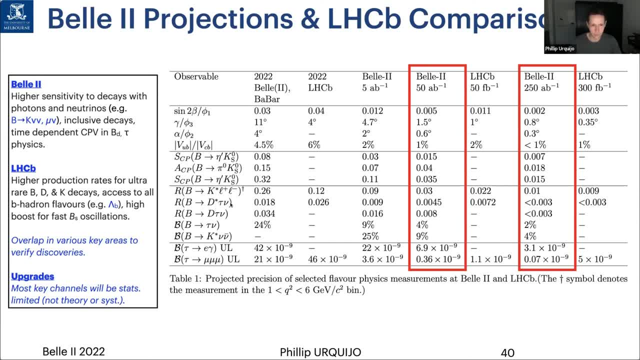 It's also the case if you're looking for channels with a, with a tau in the final state. I'd say generally we should have better prospects for precision. But you know LHCb has done very well on this channel. 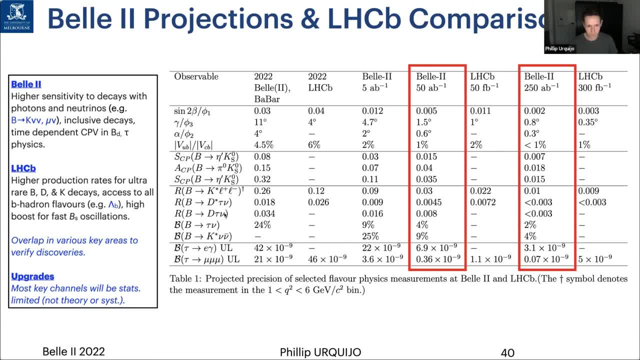 Haven't seen anything on this one. There's maybe not enough constraint And there's inclusive channels. I didn't in this table emphasize this so much, But inclusive decays means that we look at some of exclusive hadronic final states that through. 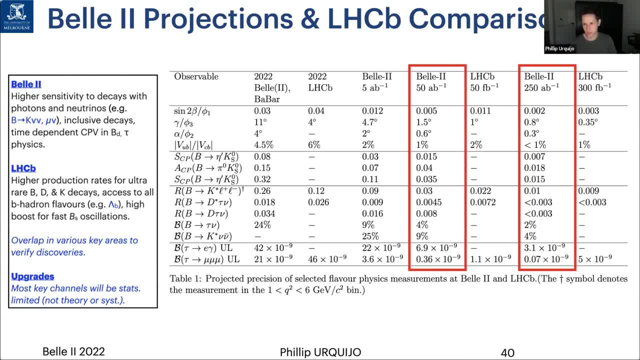 essentially quark-hadron duality effects. you can describe the transition as a quark-level transition, And so you use a different theoretical approach, And you can do that in a, in a b-factory, because you can either sum up many states or you can inclusively reconstruct, like we do for VU-B. 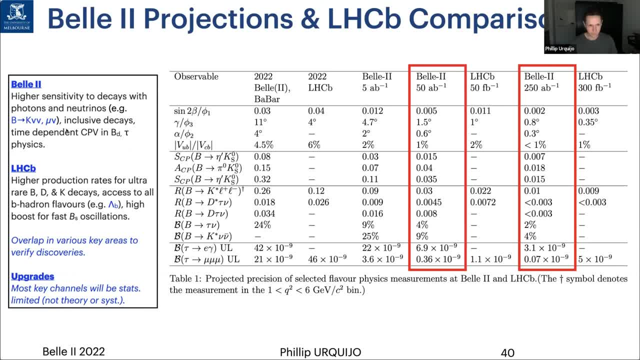 That's almost prohibitive in LHCb. Then there's time-dependent CP violation, which kind of is, I think, a little bit of a surprise, in that the fundamental requirements are that you have a good precision measurement of of delta, z And flavor tagging. 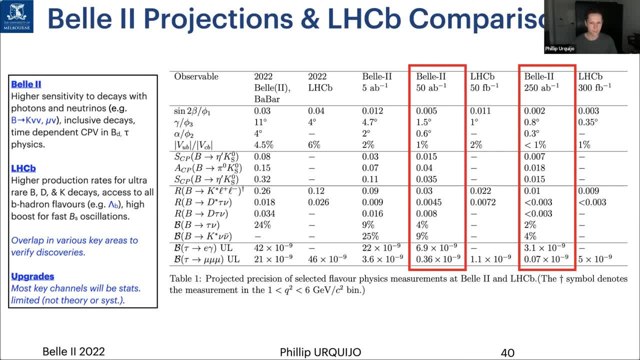 And LHCb's flavor tagging isn't as good, but it doesn't account for it, doesn't? it's not? it's essentially compensated. usually it should be compensated by the much larger production fractions. So it's the precision. there turns out that it's slightly better in the case of. 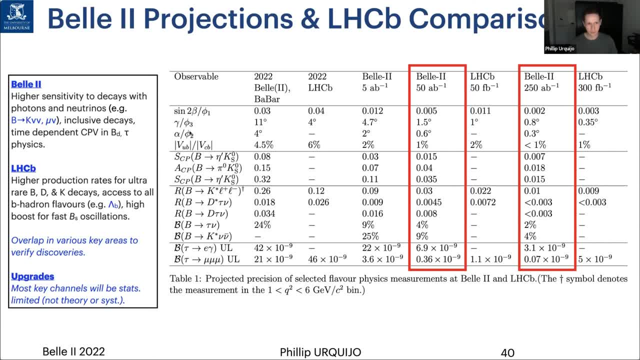 of Bell-2 for the channels that we use from B-sub-D Because of the presence of presence often of a k-short and that tends to fly out of the acceptance of LHCb. And then tau physics generally is stronger On LHCb. of course. they've got very high production rates. They've got access to B-sub-S, lambda-b. 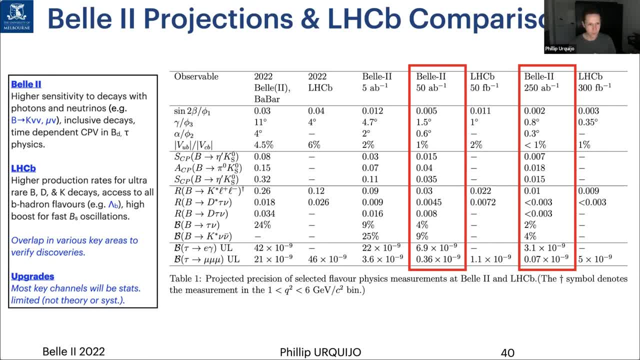 They can look at k-under-k. So they've got all that hadron flavors, They've got a huge boost. so they can measure fast B-sub-S oscillations. They can measure very rare decays as well. So B-to-mu-mu, B-to-pi-mu-mu. 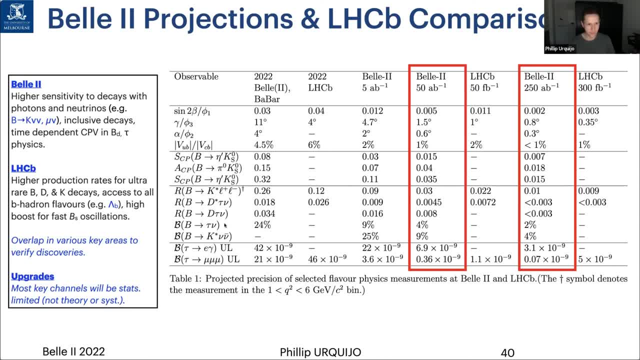 They've definitely got a very strong advantage there. There are areas of overlap that are quite interesting. One of them, I think, is k-star LL. They're past us now, of course, But the precision test that we need to do is in the electron channel, and that's where. that's where 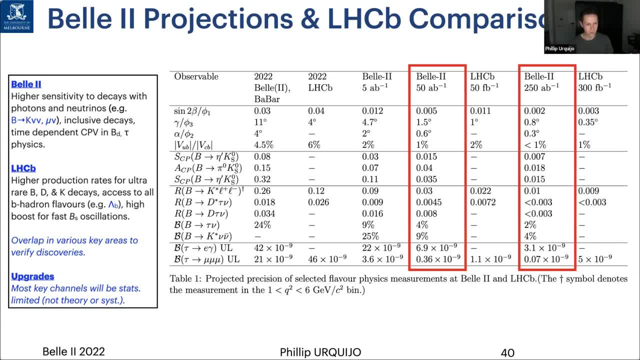 they've got more data, but we've got better resolution, so it's really nicely complementary. Yeah, I think that's the loop. Let's see there is no LHCb entry for alpha-phi-2.. Yeah, that's because they don't provide enough information for an independent extraction of that parameter, so I've not put it in the table. It would have had to have utilized other inputs directly from B-factories. 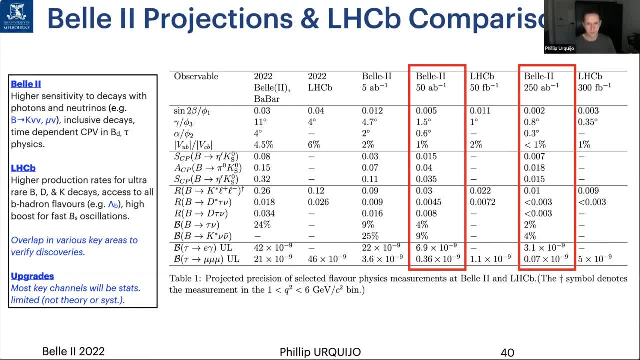 But that's not to say they're not providing input, it's just, you just can't use it alone. So maybe a star. And for k-star nu-nu-bar, does that include the latest ROE tagging methodology in the sensitivities? 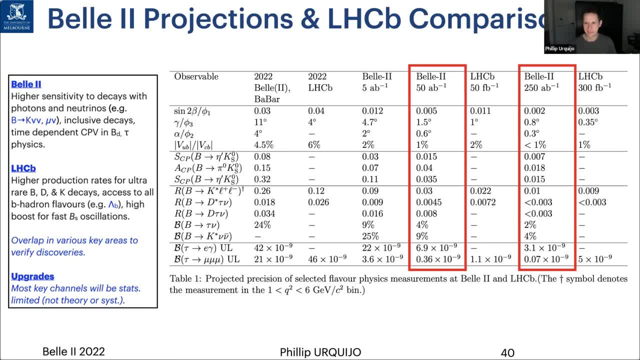 That one doesn't not yet. Yeah, Okay, so they may be even better. Yeah, yeah, definitely could be. I mean, the current one is definitely a lot more powerful. Yeah, definitely could be. I mean, the current one is definitely a lot more powerful. 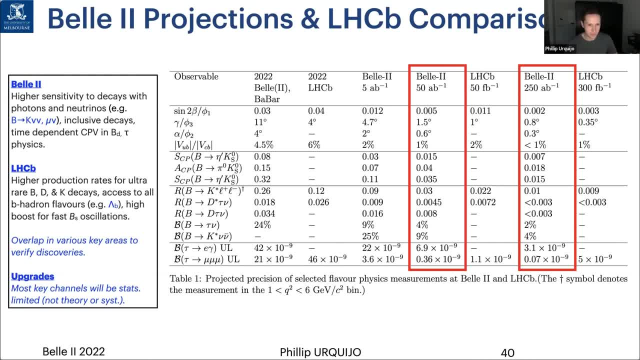 Yeah, definitely could be. I mean, the current one is definitely a lot more powerful. But I guess after that first publication- now we've got a lot more data that is being studied- we'll have a better handle on perhaps the systematic errors and potential bias in a more inclusive approach and that makes it easier to extrapolate.